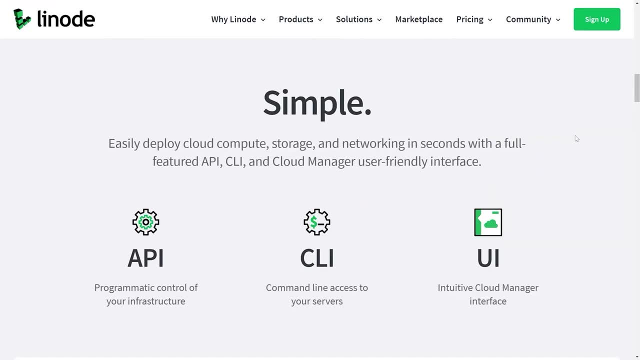 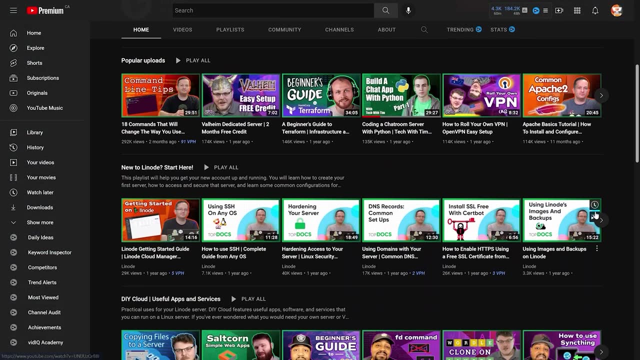 new data centers around the world in the near future- Next year. Linode makes it super easy to spin up service with their one click app marketplace and have tons of written guides and YouTube videos on their channel to help you get started Now. if you're having any issues, you can reach out to their 24 seven support team and 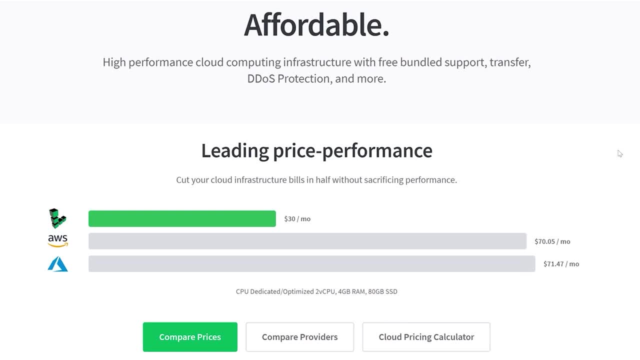 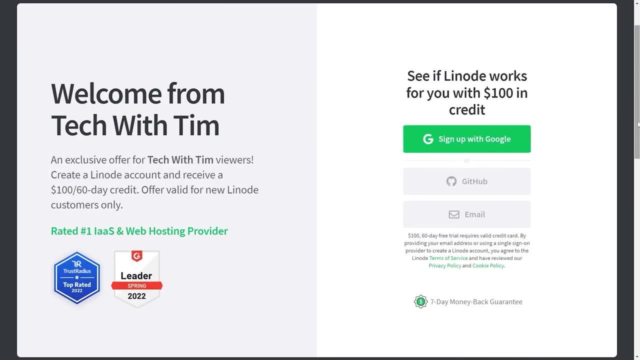 actually talk with a real human being. Now Linode's pricing is simple, with no hidden fees and full transparency, and you can test out Linode services for free by using the link in the description and claiming an a hundred dollars 60 day credit for any new. 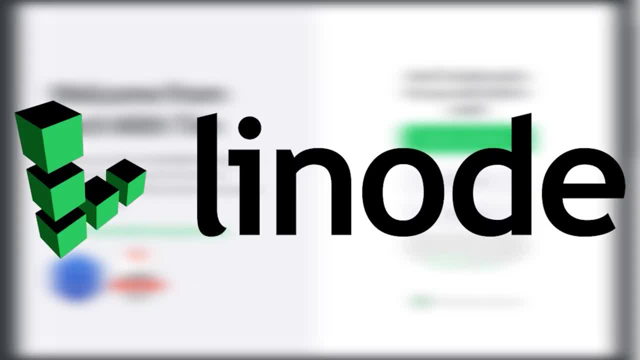 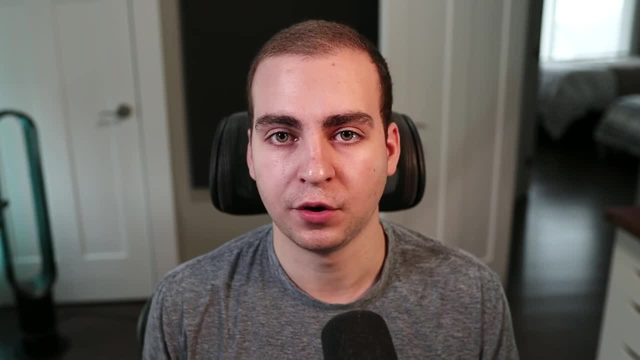 accounts. It's been an absolute pleasure to work with Linode over the past few years. I've been working with Linode for a few years, and one last thank you to them for sponsoring this video. All right, So let's dive into this project. I just quickly want to mention, if you don't, 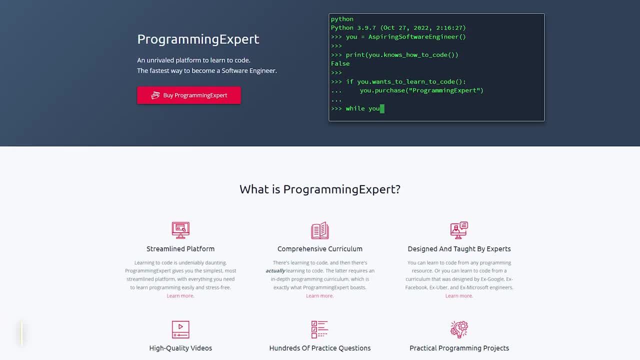 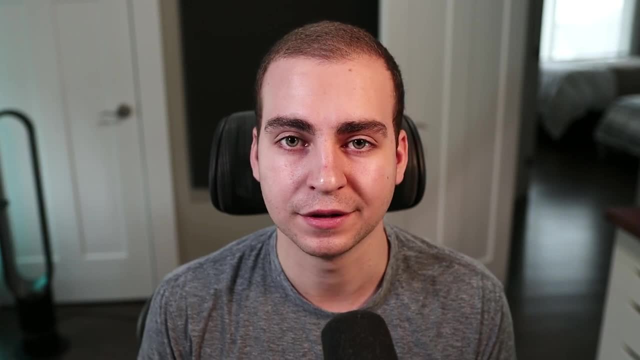 already know, I do have a programming course. It's called programming expertio- great place to become a software engineer and learn how to code specifically in Python. and go check it out. If you haven't already, I'll leave a link in the description. All right, So let. 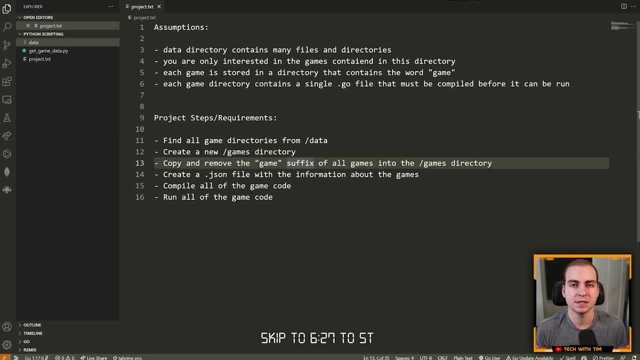 me start by walking you through the project that we're going to complete. Now, this is a project that kind of mocks what you would be doing in a real world scenario. Obviously, I don't know what you guys need to automate or what sort of stuff you guys need to automate. So let me start by walking you through the project that we're going to complete. Now, the project that I'm going to complete is called lay down the crap script. You can see that you name it and actually it's going to show you exactly what it actually says. 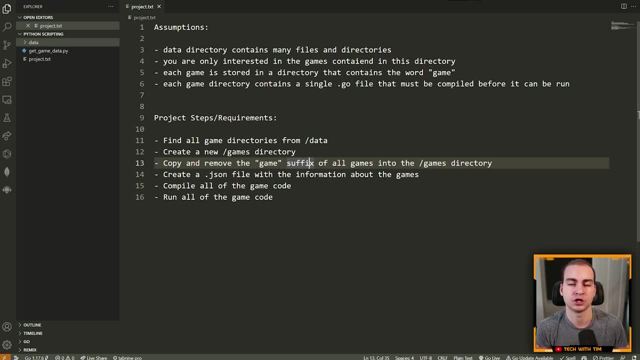 So here's the code that we're going to use to create the script that you need to write. So I've tried to create something that's very general, that allows you to get a bunch of knowledge in a ton of different areas, So this may not cover everything you need to. 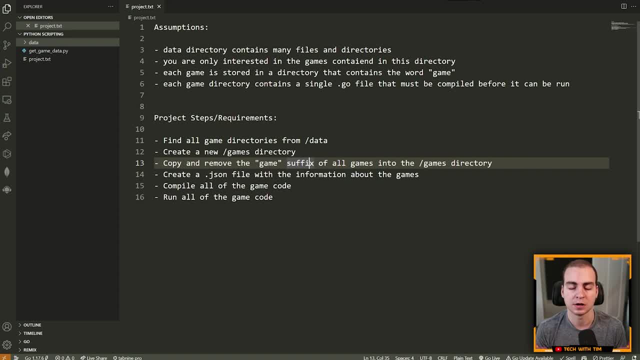 do. but it will give you a ton of that base knowledge and show you what's possible with Python scripting and how you can kind of set up these scripts to be as effective as possible and what commands you should be using for a lot of the common operations. So let's have 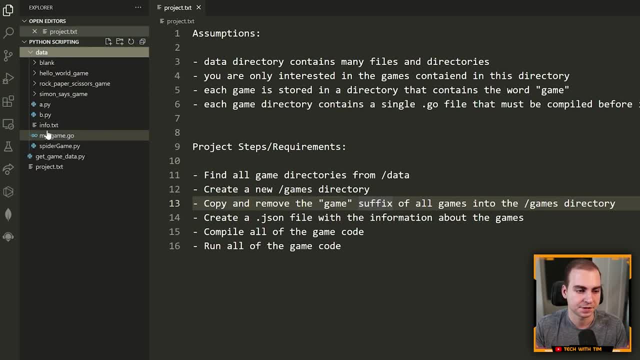 a look at it here. First thing that I want to look at is just the directory I have on the left side of my screen. Now you guys can download this by going to my GitHub. I will leave a link in the description, of course. 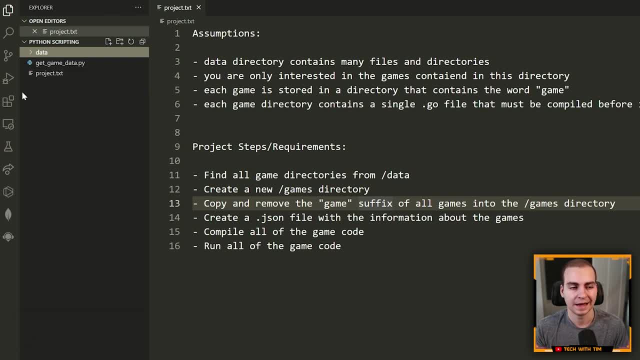 and just clone the repository, download the repository and get access to this data directory here. Now this data directory is going to kind of simulate kind of a large project, some code or some files that you would already have and that you want to traverse through and do. 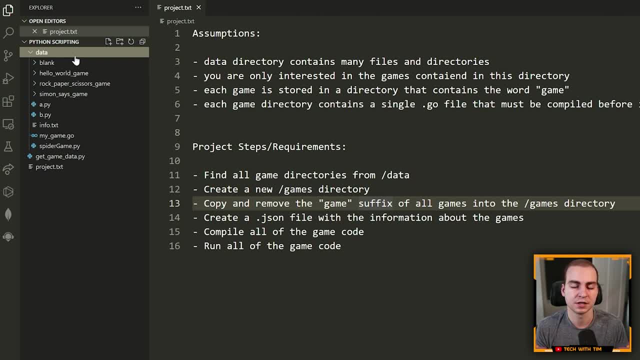 something specifically with. Now that's usually what automation is or scripting is. for me in Python, It's going through some existing data or an existing file structure and kind of parsing things out, grabbing specific data, looking for certain names or writing code into different files. So 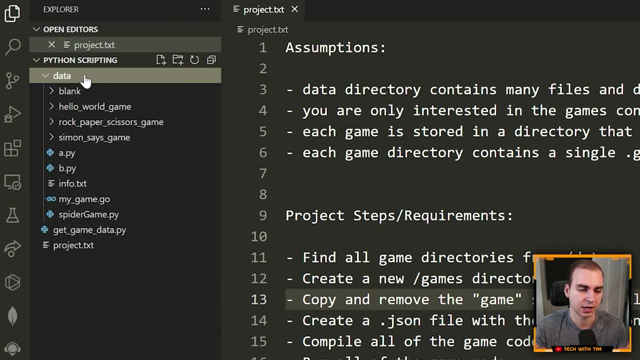 I've tried to kind of emulate that here So you can see we have this data directory here and inside of here I have a bunch of stuff right. I have some empty directories. I have some directories that are representing kind of games that would be. 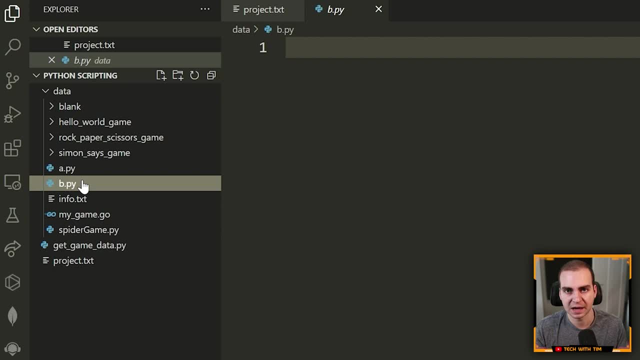 written in go. I have some random Python files. They're just empty, Just for example purposes. I have a text file, I have another kind of go file here and you can see that there's a bunch of stuff in this directory Now. 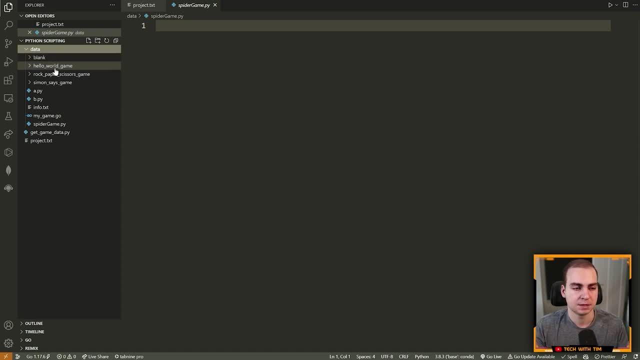 what we're interested in here for this kind of mock project is parsing out all of the game directories. So what we want to do is want to take all of the games that are inside of this directory. We want to copy these into a new directory. We want to. 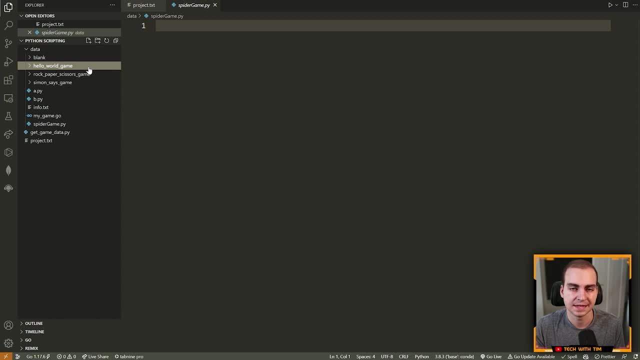 change the names of the directory such that we don't have this game kind of suffix on them. And then we want to compile all of the game code that exists inside of these game directories. And this is something I actually had to do when I was working. 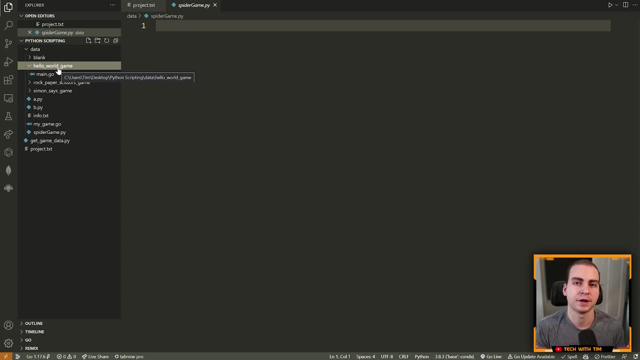 for my startup, as I mentioned in the intro. So I've kind of put a variation on it here. Now, to go even a step further: once we get all of this game data, we parse it out, we put it into a new directory and we 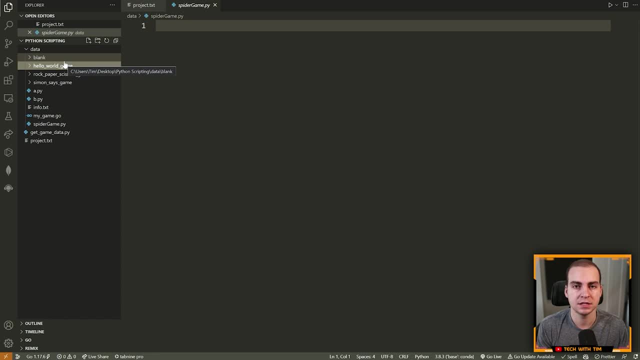 compile all of the code. I want to write a Jason file into that directory. that gives us some metadata or information about what we just did. So how many games are there, What are the name of our game directories, et cetera, And that's. 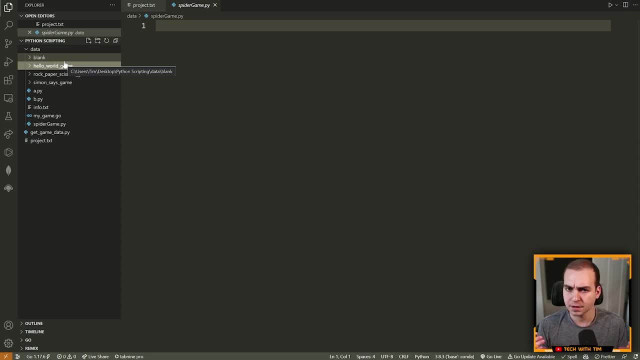 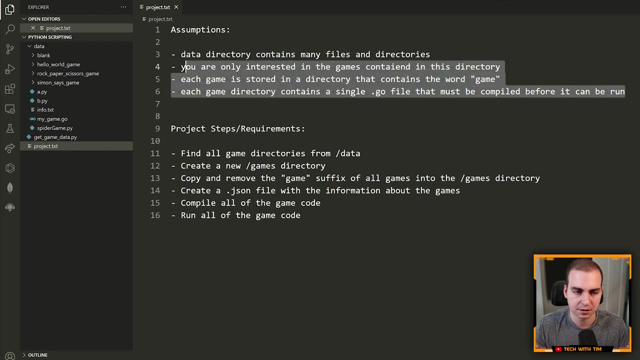 something that we could kind of quickly look at to get a summary of the information So you can imagine. this would be something similar to what you may want to do when you are writing your own Python scripts. Okay, So I have a kind of the 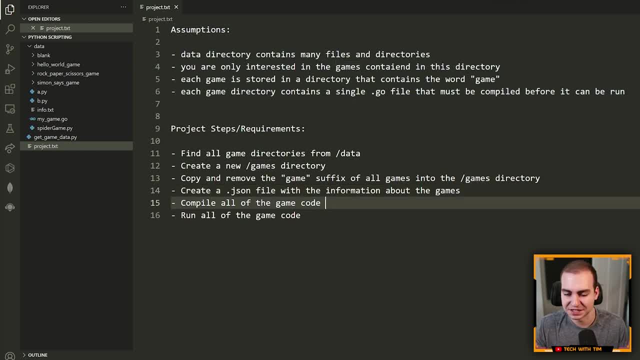 project text here. excuse any spelling mistakes that are in this file, but I just wanted to walk you through very organized, step-by-step, what we're going to be doing. so much So some assumptions here. sorry, uh, the data directory contains many files and 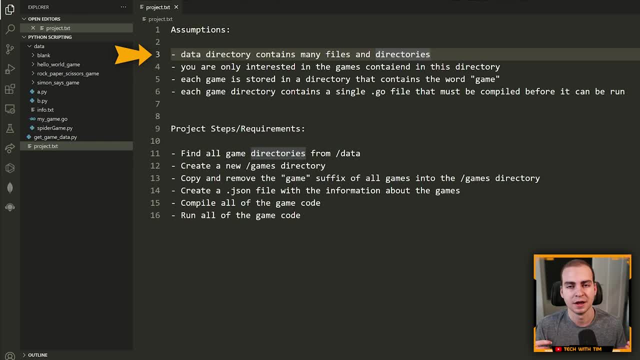 directories. So imagine this is massive, right, There's a ton of different code in here and it's not feasible for us to do this manually. We want to have a script that automatically does it for us. Obviously, that's not really the. 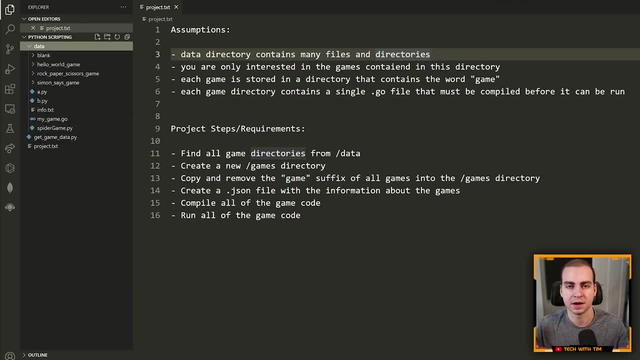 case here, but again kind of picture that we had, you know, thousands of files. in that case, it would be very helpful to have a script to help us do this. You are only interested in the games contained in this directory, So 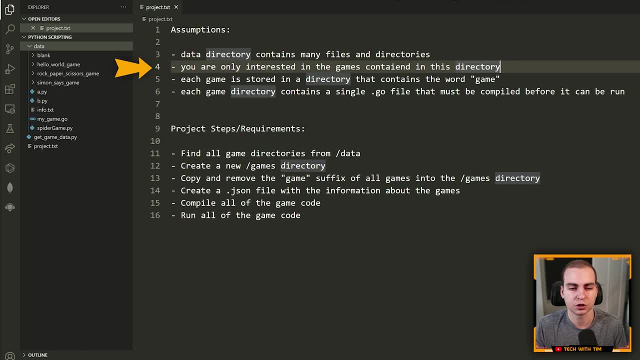 So you don't care about the rest of the junk in there, You just want the games which are going to be stored in a directory that contains the word games. So whenever we see the word game and that's in the directory name that we 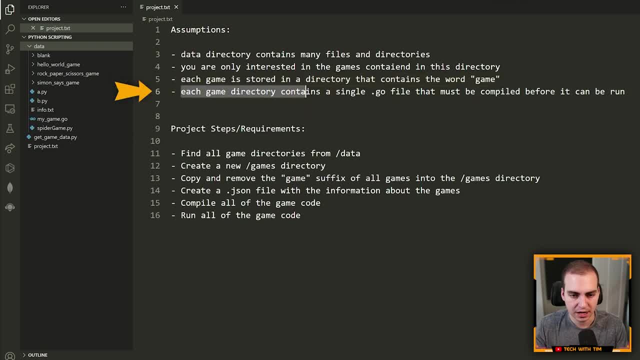 know that we're interested in that directory. next, each game directory contains a single doc go file that must be compiled before it can be run. Okay, perfect, That makes sense. And these go files could be named different things. Notice one is called. 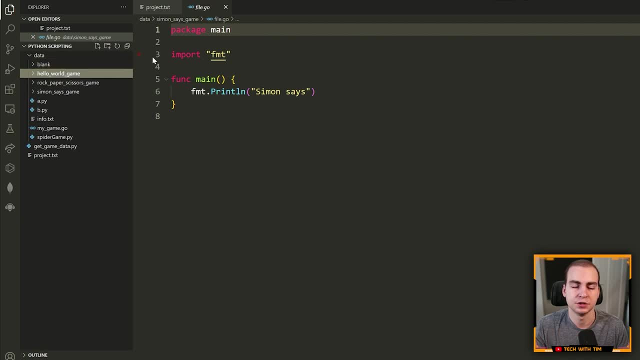 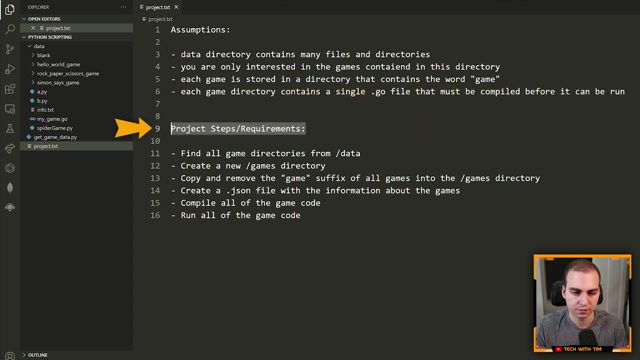 main. one is called code, One is called file. So we're going to have to do um kind of special stuff to handle these different names and compile all of this code. Okay, So now, what are we going to do for this project? Well, we're. 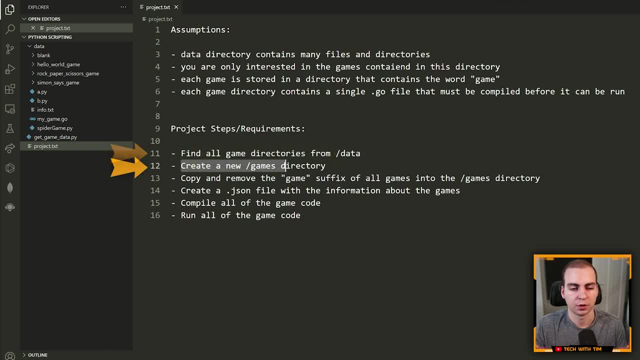 going to find all of the game directories from the data directory. We're going to create a new slash games directory, or whatever we want to call it. That's going to contain all of our game code. We're going to copy and remove the game. 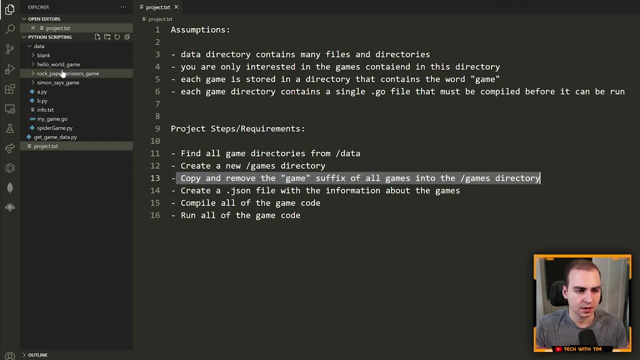 suffix of all of the games into the games directory. So that means copy the directory, strip off that kind of game aspect of it, put it into the new directory. We're going to create a Jason five File with the information about the games. So how many? 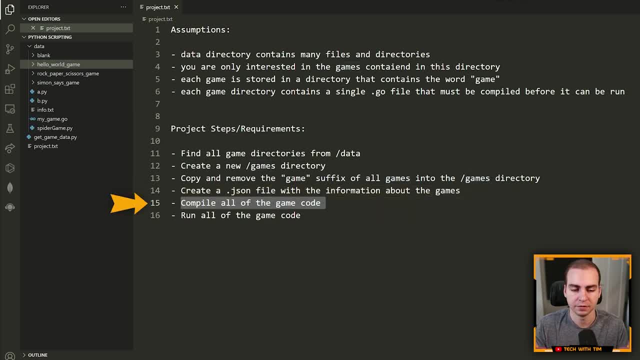 games, what the game names are, et cetera. We're going to compile all of the game code and then run all of the game code. Now, we may not actually run it here, but we will at minimum go to the compile step. 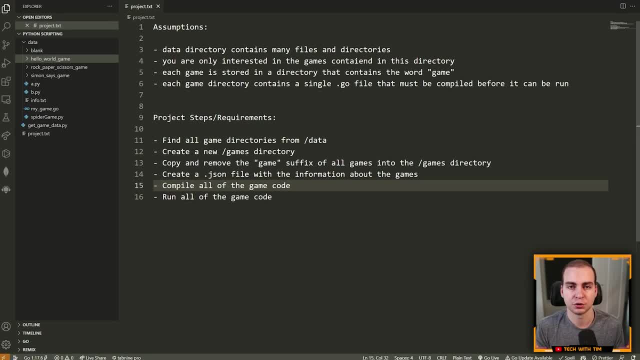 Perfect. So the only thing we need to do here to get started is make sure we have Python installed. I'm going to be using Python 3.9,, I believe, but I think anything above 3.8 should work, And if you. 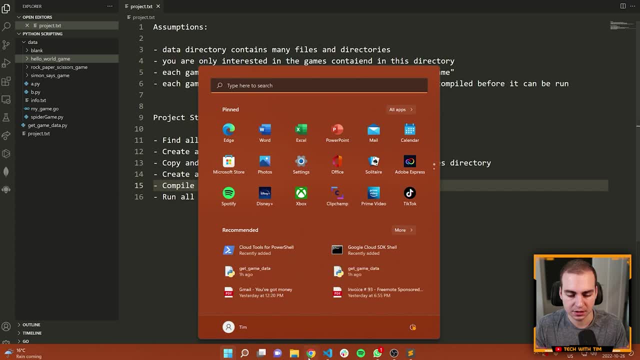 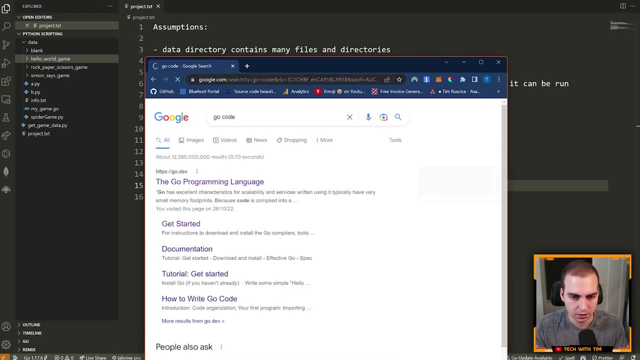 want to be able to compile and run this go code, then what I'm going to suggest to you is that you download a go um interpreter or compiler. So let me just bring this up here and go code. I'll leave this link in the 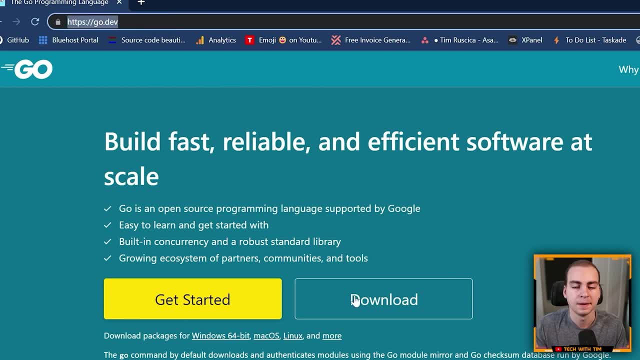 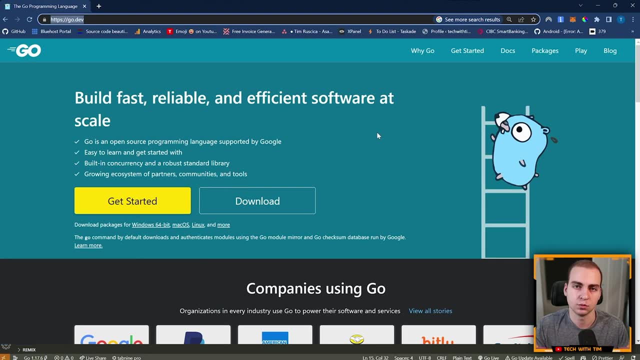 description as well. But if you go to go dot dev- pretty simple URL, click download. it will download and install go. It will automatically add it to your path. Then you'll have access to the go command that we'll be using later in the 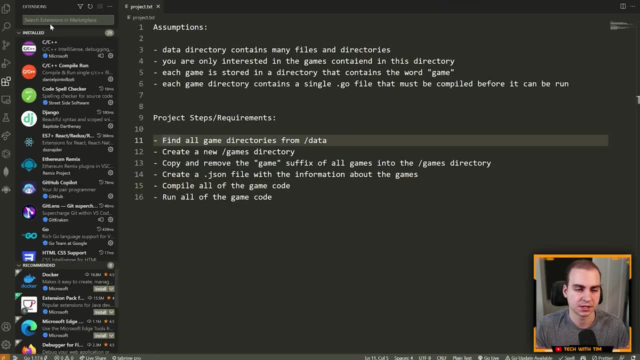 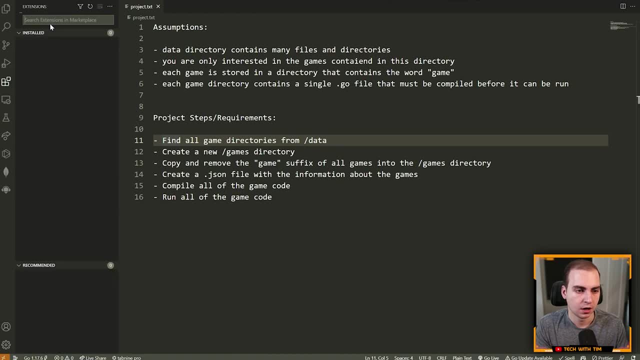 video. Last thing, if you want, there's some helpful extensions here in VS code. If you're using VS code, you probably want to install the Python extension and the go extension as well. Okay, So let's go. So, now that we've got, 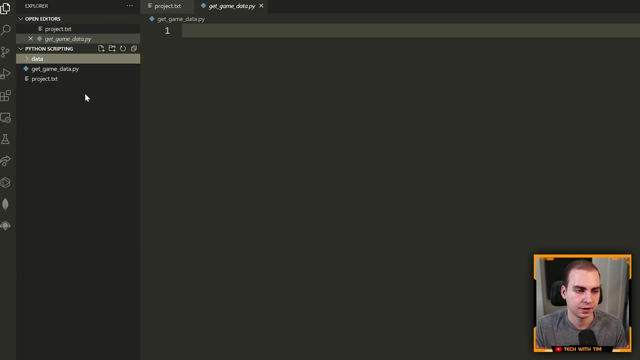 through that, let's start writing our code. So I have a Python file here called get game data. You can call this whatever you want and notice I've put this in the same directory as where my data directory is. that you don't need to do that, but it is. 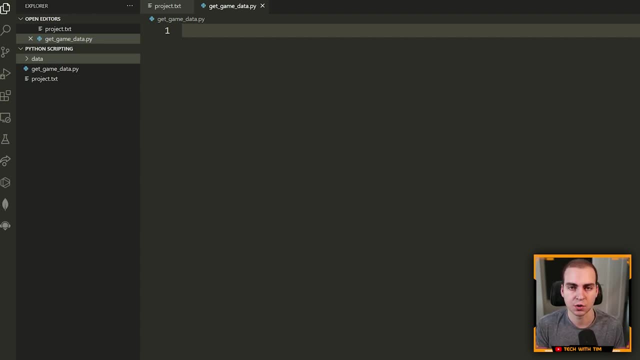 going to be helpful to have it kind of close to the data directory So you know the path to where that is. So again, if you want to go to the GitHub, I'll leave that link in the description. download this code It. 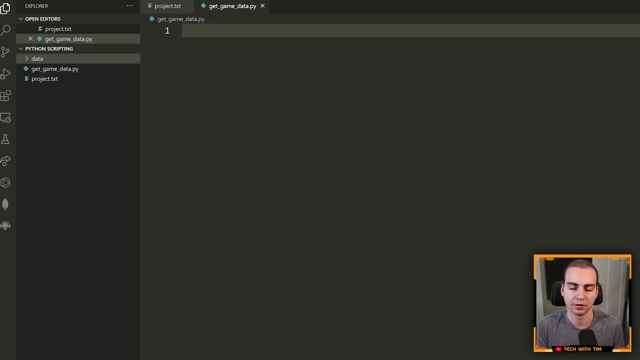 will have the finished code as well, but you can just kind of delete the file and write it along with me, if you want, And then you'll have the go to the this data directory So you don't have to kind of create this on your. 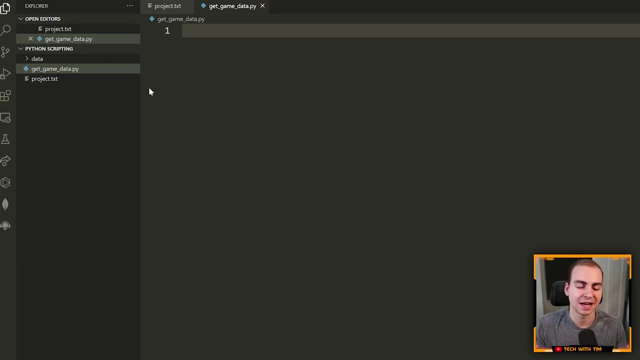 own. So you want to work in a Python file that is in the same directory as the data directory, And the first thing we're going to do here is just import a bunch of modules that we're going to be using. So we're going to import the OS. 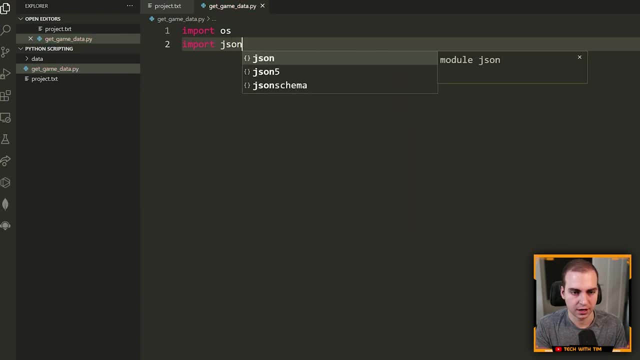 module, which I believe stands for operating system. We're going to import Jason, which is how we're going to work with Jason files. We're going to import S H, U till uh, which is going to allow us to kind of do some copy, and 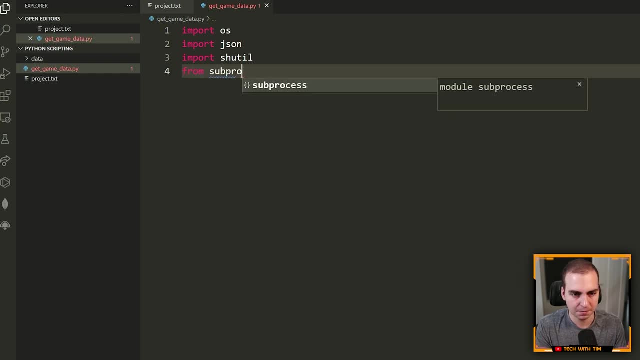 overwrite operations. We're going to say, from subheadings, we're going to sub process, import, and we're going to import pipe and run. Now this is going to allow us to run really any terminal command that we want. So we can, for example, 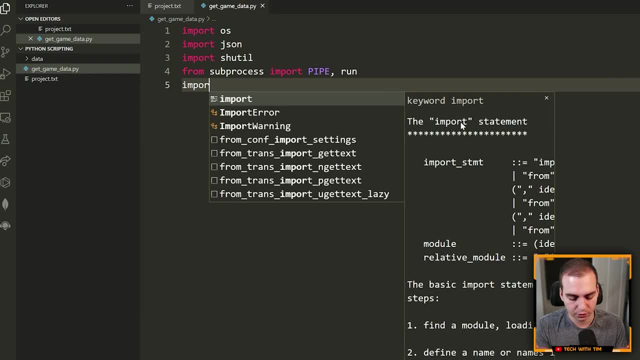 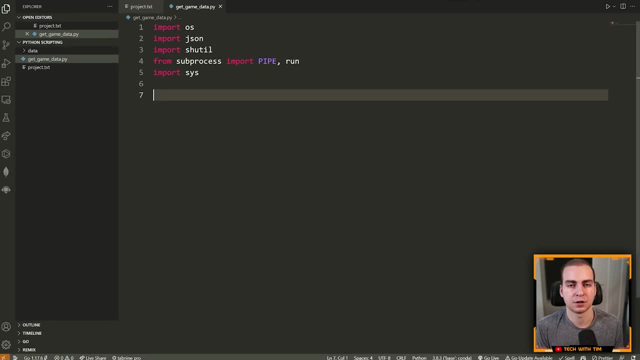 compile and run the go code using this, And then we are going to import S Y S, which we are going to use to get access to the command line arguments. So the very first thing I want to start by doing here, if we go back to our 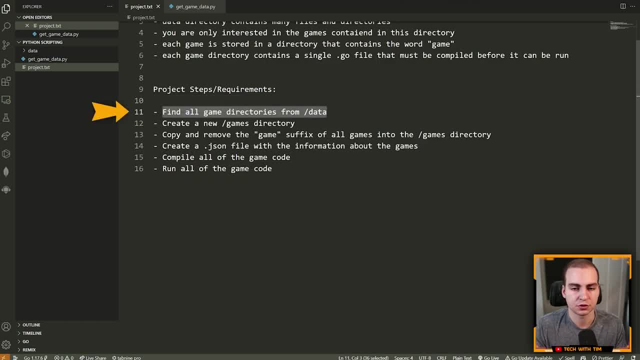 project text is: we want to find all of the game directories from some directory. In this case is called slash data. We want to create a new directory, some kind of target directory, or we're going to be copying this into. So what I want 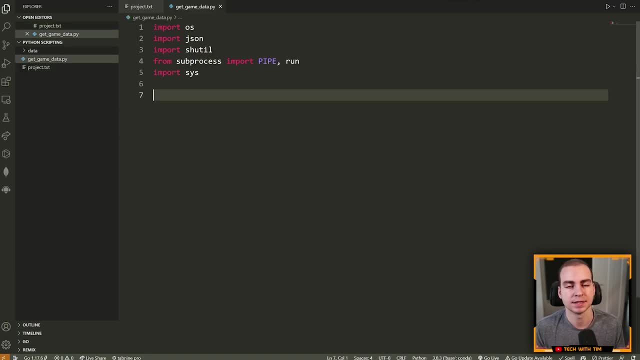 to do is I want to grab from command line arguments what the source directory and the target directory is relative to the current path, so that I know where I should be storing kind of all of the games that I find and where I should be looking for those games. 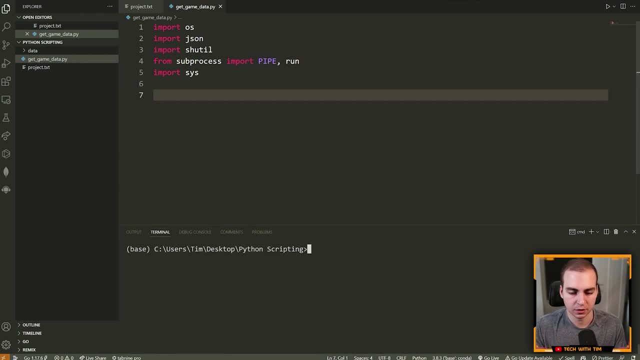 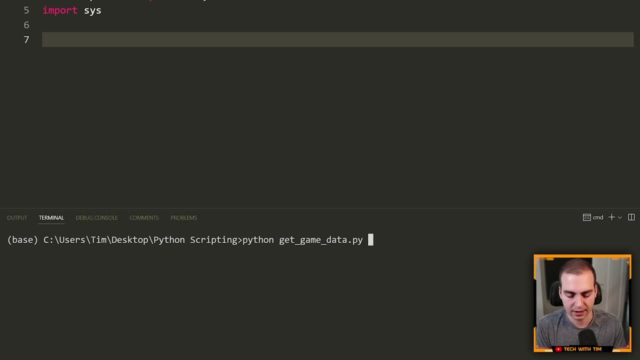 to make this script a bit dynamic. So what is the command line argument? Well, let me just show you down here in the terminal. So command line argument is something like Python: I pass my app file name So it'll get game data, And then 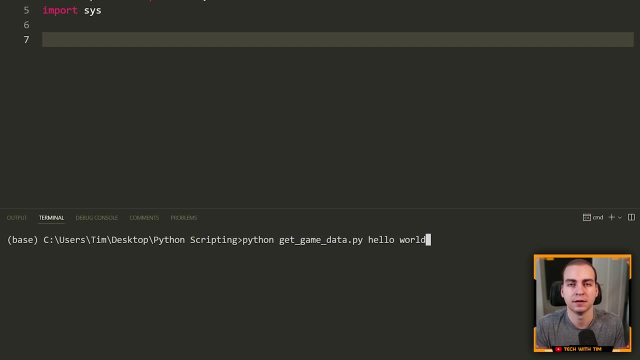 I do something like hello, world. Okay, So hello And world are command line arguments. You've seen this before. whenever you've ran any commands, like when you make a folder MK during- then you put the folder name. the folder name is: 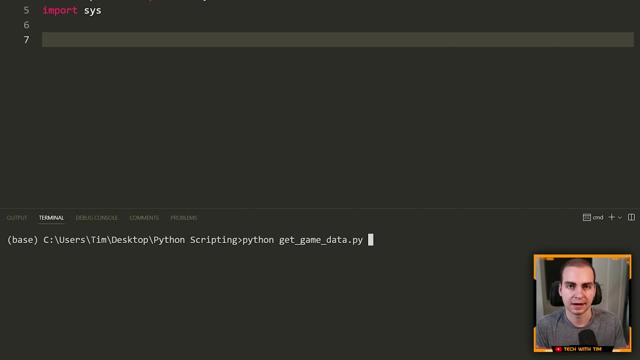 a command line argument. So in this case we might do something like Python: get game data, that we pass slash data, which is going to be our source directory, And then we pass something like slash new games or something like that, And that's our output. or 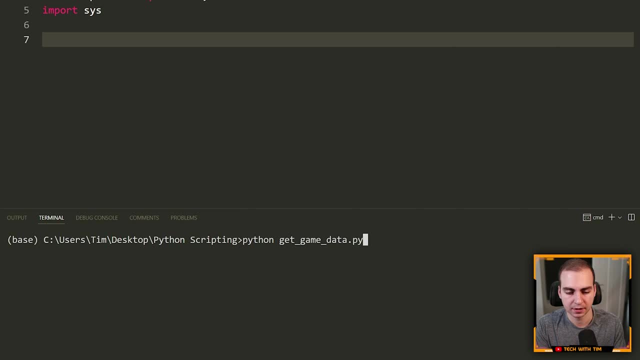 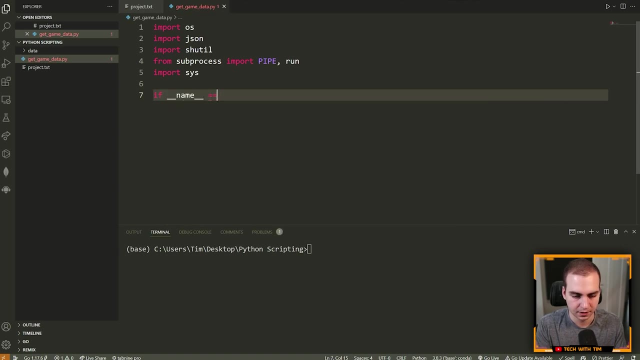 target directory. So I want to show you how we can parse out those command line arguments. So to do that we're going to use the system module. So first I'm going to say: if underscore- underscore name is equal to underscore underscore main, then in here I'm 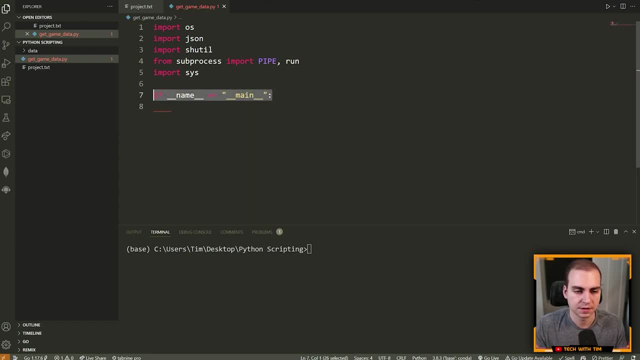 going to grab the command line arguments. Now, the reason I'm using this is because I only want to execute the main script here. If I'm running this Python file directory- uh, directly. sorry, if I'm not directly running this Python file, I don't. 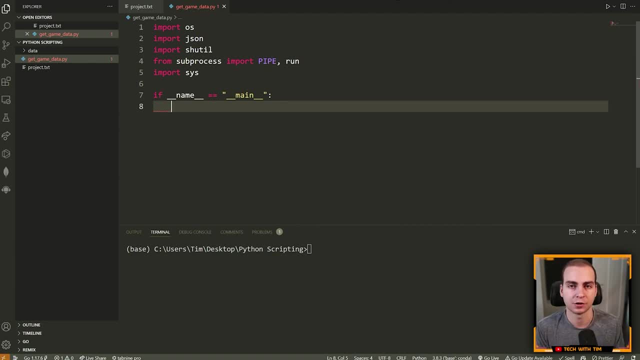 want to be executing the code That's going to run through and do all of our operations. Uh, otherwise, if we tried to import the Python file and we didn't have this line, it would go ahead and run all of that code when we don't. 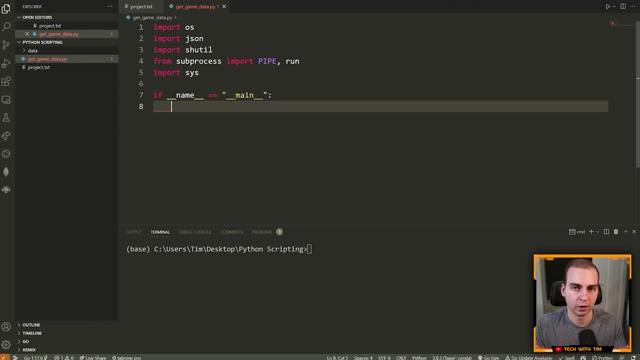 want that to happen. So when you have this here, this just checks that you ran the file directly and it won't execute anything in here If you were importing, say, a function or a class or something from this file. hopefully that makes sense. What? 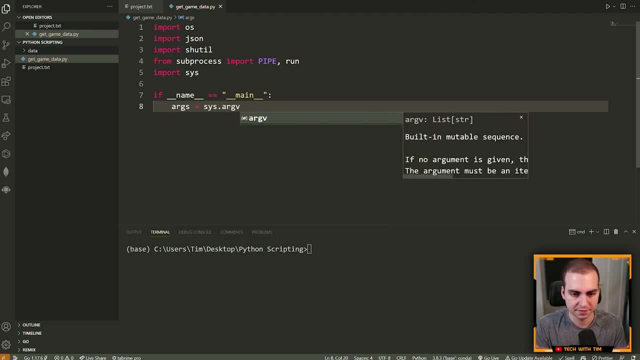 we'll do here is say: args is equal to S, Y, S, dot, R, V. Okay, Now just to show you how this works, we'll print out args, uh, and let's run our code. So I'm going to say: Python, get game. 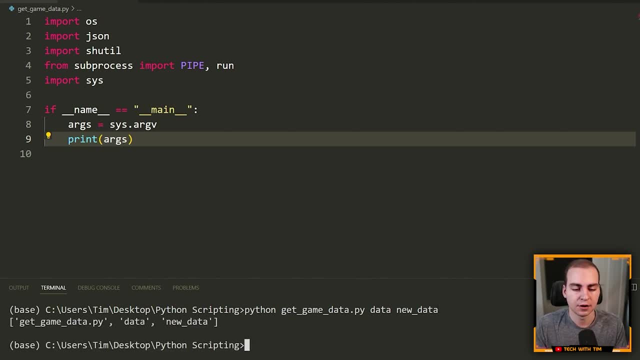 data data: data data data, new data. Okay, Hit enter And notice that my command line arguments are first of all the name of the Python file, And then I have my two command line arguments, or data and new data, that I passed here. 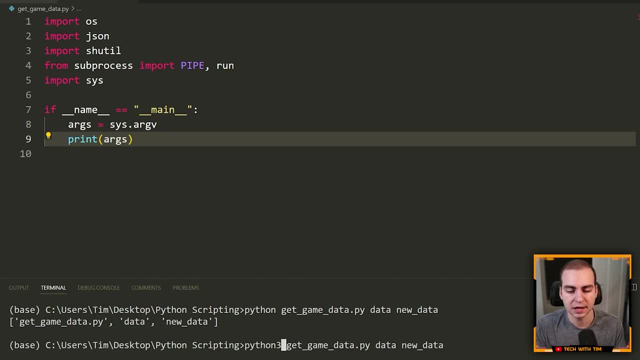 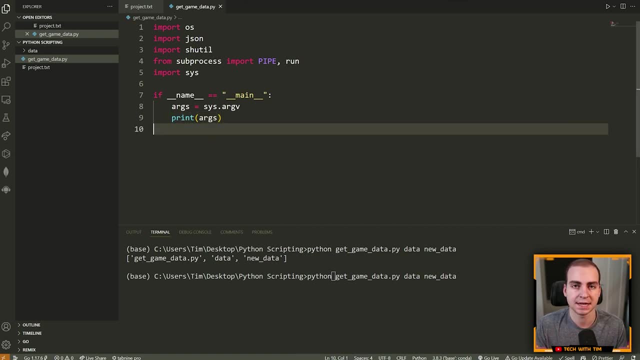 Now, if you are on Mac, you will probably need to run a Python three get game data, Okay. So, now that we have our arguments, I want to make sure that we have a valid number of arguments, which, in this case, is: 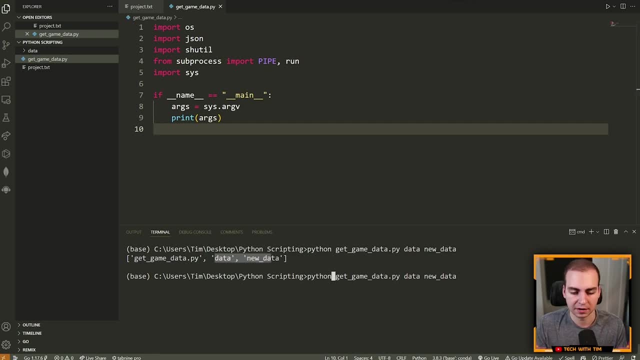 going to be three. three because we have the file name and then we have the two extra arguments and we want to make sure we have those two extra arguments. So I'm going to go here and say: if the Len of args does not equal three, 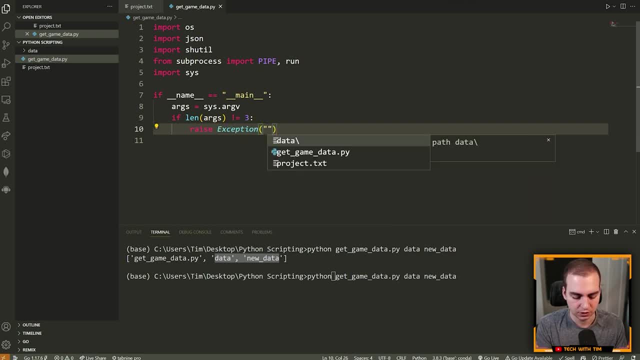 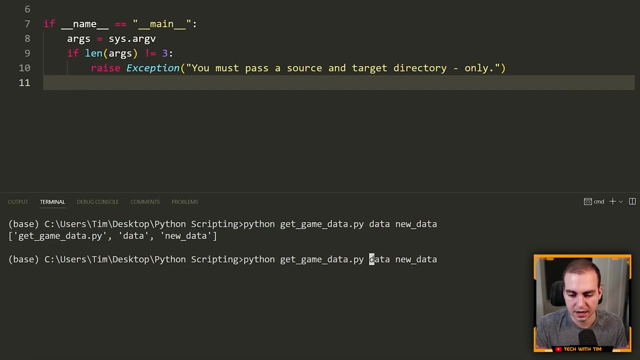 then I will raise an exception in here. I will say: you must pass a source and target directory only. Okay, So that's fine. So now, if we run our code here and I only pass, for example, the source directory, then notice that I get my 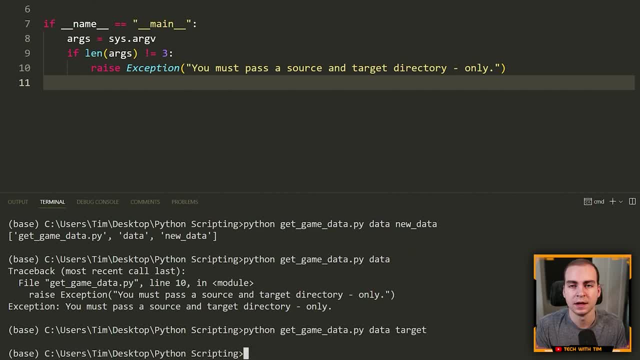 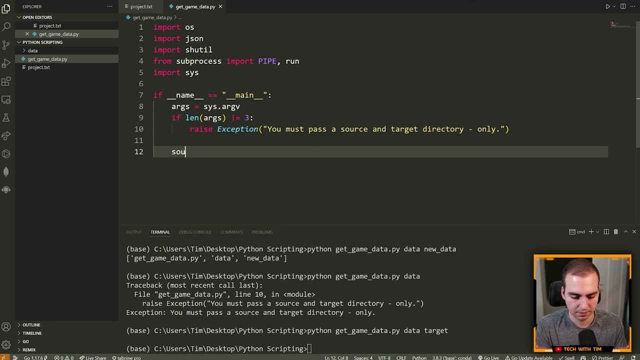 exception. If I pass my target as well, then all is good. Okay. So now I want to get my um source and target directory. So I'm going to say: source target is equal to S, Y, S, dot, R, V And. 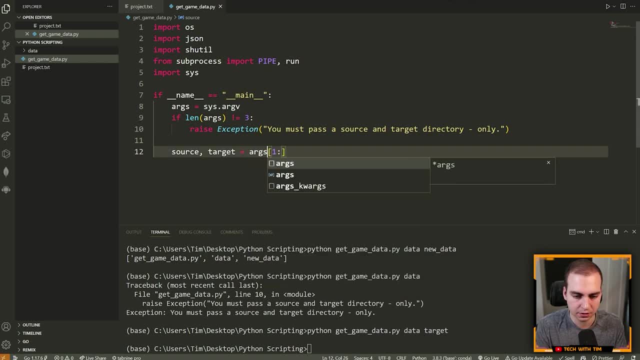 then I'm going to do one colon like this, And actually we can put this as args. Now, the reason I'm doing one is just to strip off the name of our Python file, which we don't want, and just get the two arguments here. 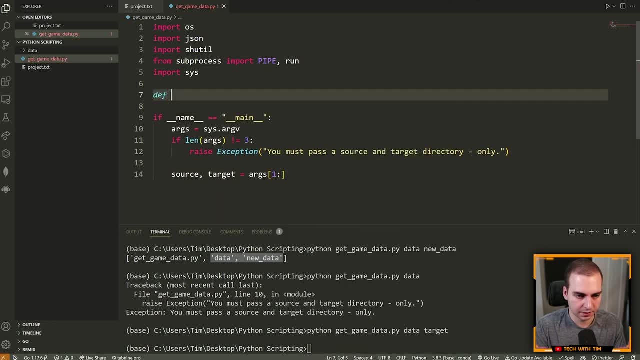 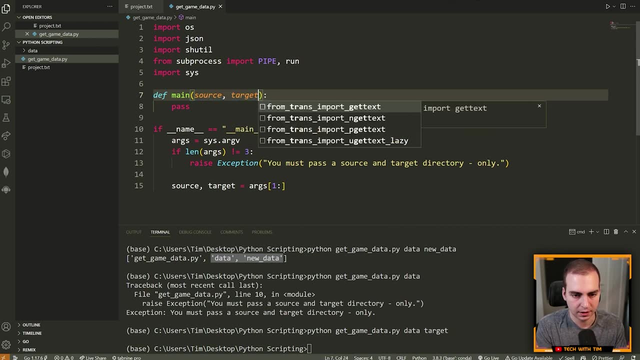 and then store them in separate variables. Okay, Now that we've done that, I'm going to create a function And this main function is going to accept our source, Okay, And our target, And I don't know if that's actually the right thing. 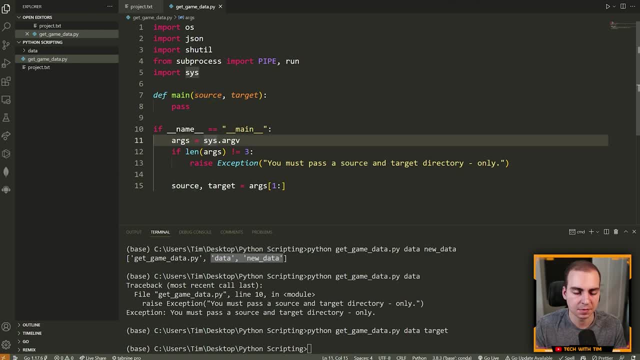 that we want to call it. Um yeah, I guess that makes sense. Sources: where we're looking target is where we want to put our new directory. So that's fine, We can leave it like that, And then here we'll go and call the main. 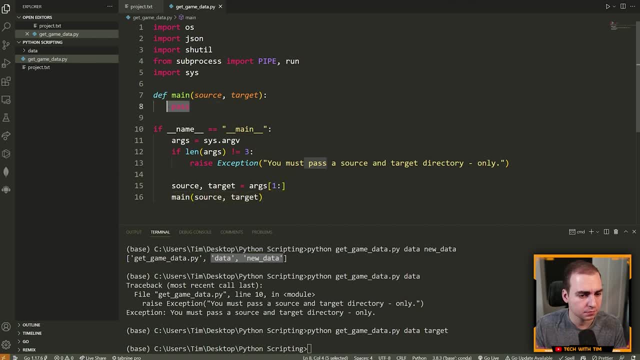 passing our source and target directory names. Perfect. Now that we have done that, what we actually need to do- is to actually need to do here before we go any further- is we need to create a complete path from the location where we're running our Python file to 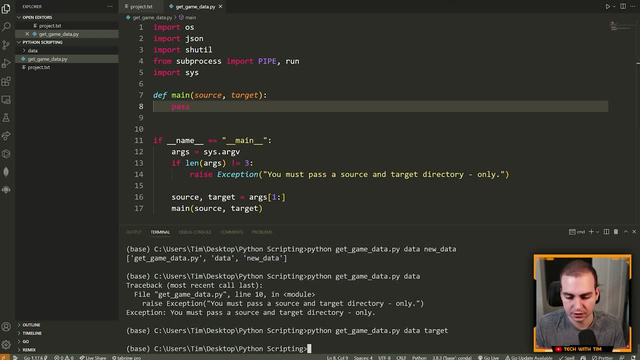 whatever this directory is. So in the case where I pass, you know, data or target, well, I want to get the full qualified path from, say, like my C drive, all the way to this directory so that it's going to work in my 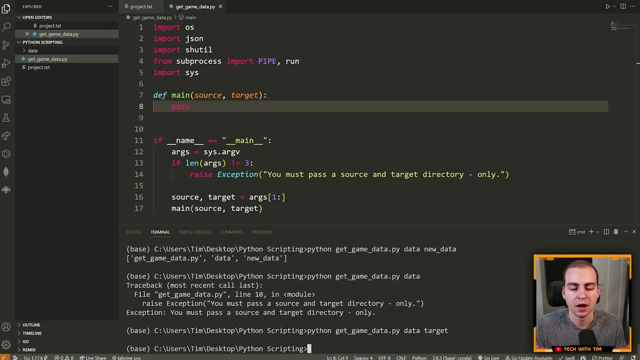 program. If I just try to use data or I just try to use target, uh, we can get some weird errors depending on what operating system we're running on. So what I'm going to do here is, say my source underscore path is equal to O S dot. 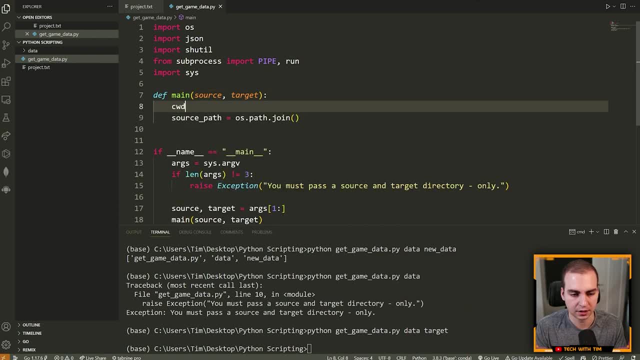 path dot join. And the first thing we need here is the current working directory, which I can get by using the command I got to check my sheet cheat sheet here, Cause I always forget O S, dot get C, W, D. Okay, So I'm going. 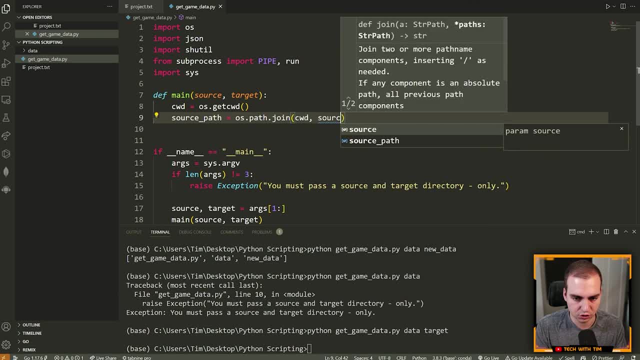 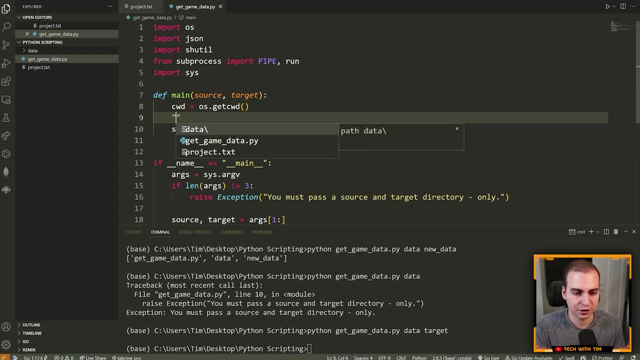 to join the path of C, W, D and my source directory. Now you should always use O S dot, path dot, join When you're trying to create paths. don't think you're going to be clever here and have a path, Like you know, C drive. 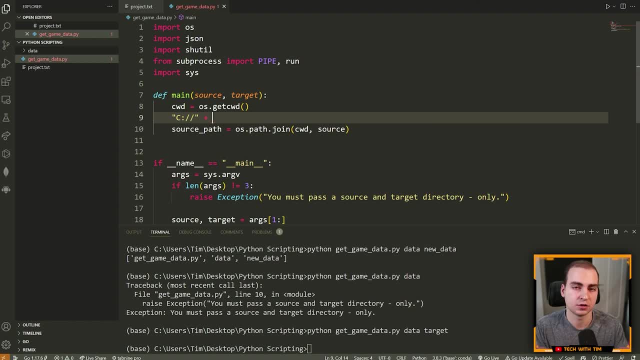 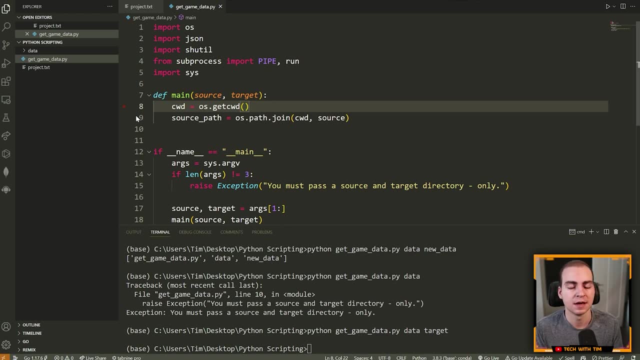 colon, slash, slash, and then you add, like you're doing a string concatenation. Don't do that. The reason you should not do a string concatenation is because if you're working on different operating systems, the path dividers are different. When you 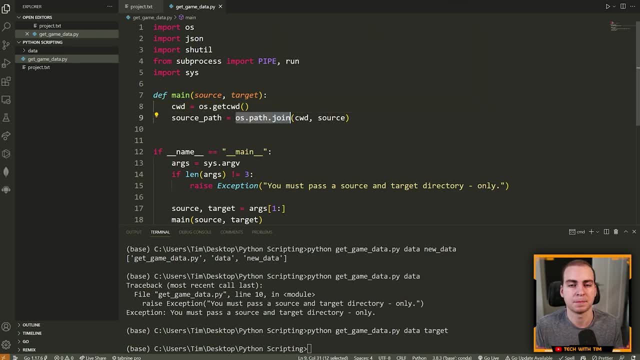 use O S dot path dot. join it automatically will join the path based on the operating system you're working on. So you always want to use this. Don't do string concatenations, uh, to try to create paths. It might work sometimes, but it's. 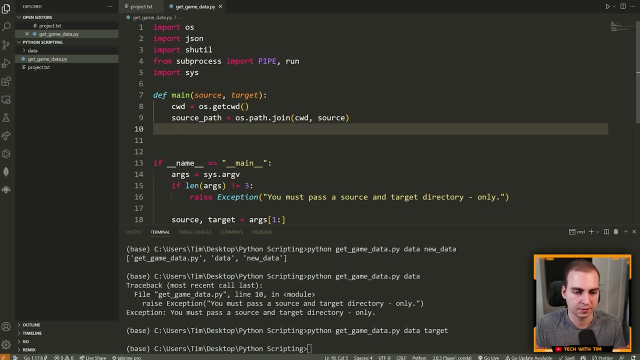 not kind of a good practice to do that. Okay, So we've created our source Path. Now just to explain this line here: CWD is our current working directory, which means the directory we ran this Python file from, So wherever we ran, 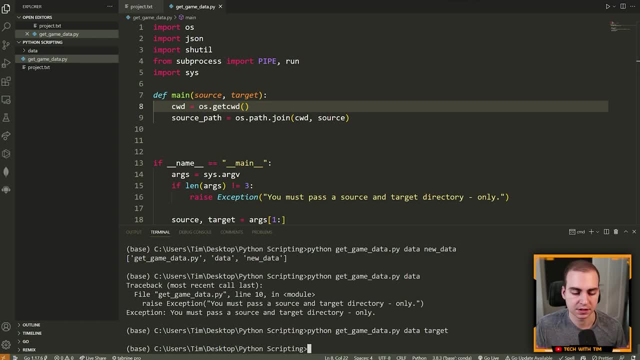 this Python file from: uh. that's the working directory, So in this case it's going to be users Tim desktop Python scripting. then whatever these paths are are going to be relative to that working directory. So I combine them together, right? So? 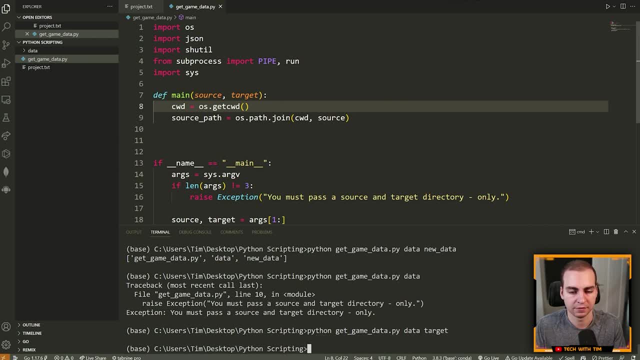 now the directory will be this and then it will have my source, which would be data right, And then the next one will be my target. Okay, So let's copy this and make this target and change this here to be target. Okay, So now we 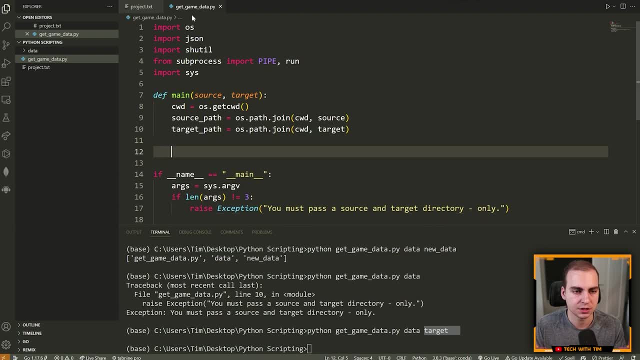 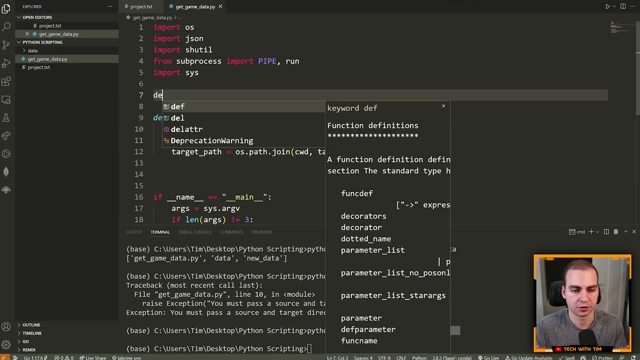 have our source path and our target path. Now what do I need to do next year? Well, I need to find all of the game directories from my source directory. So let's write a function that can do that. We'll say: find all game. 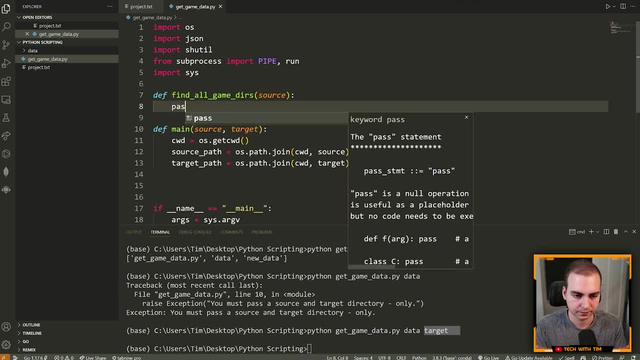 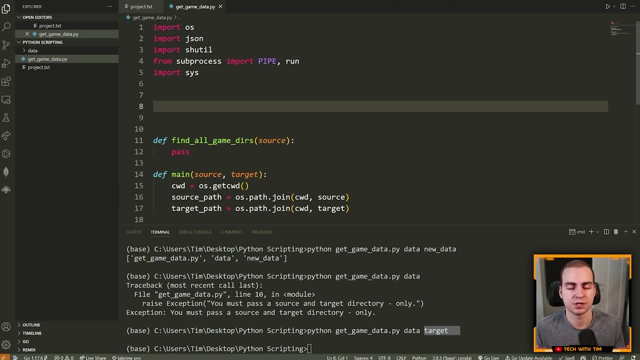 doors like that. We need to know where to look, So we'll go source. Okay, I'm going to create a variable up here and this is going to specify what we're looking for in our directory. So like what needs to be in. 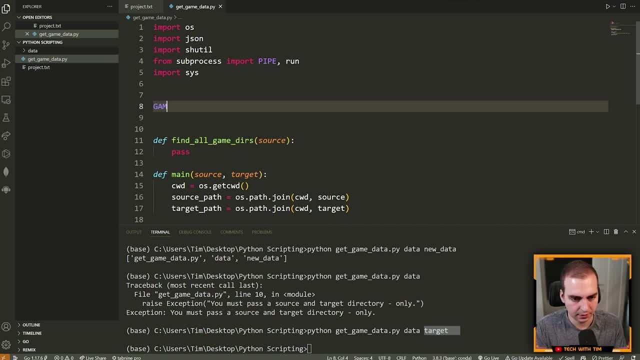 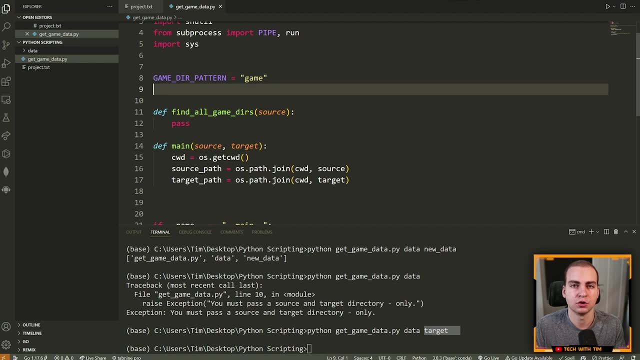 their name. So in this case I'm going to say game. dirt pattern is equal to, and we'll just call this game, which essentially means we're going to look for the string game in any directories, Uh, and that will tell us that we want. 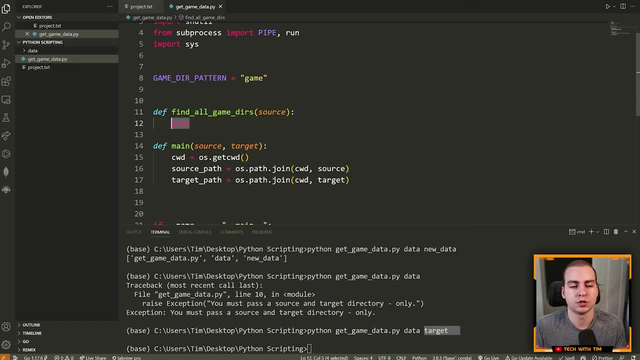 that directory right now. what we're going to do is we're going to essentially walk through the source directory, look at all the files and directories and then match any directories that have a game in them, Um, and if we have that, then we'll. 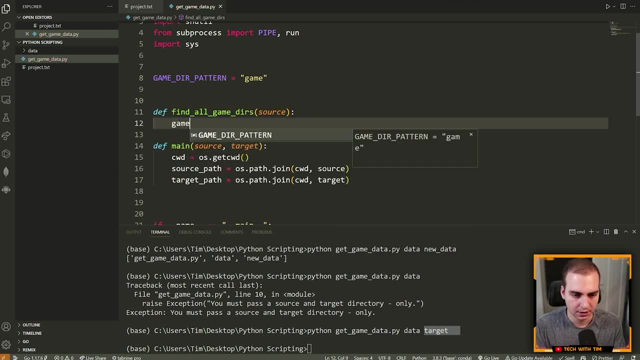 add them to a list, We'll return them, et cetera. Okay, So let's do this. I'm going to say my game underscore paths is equal to, and this is going to be a- uh, what do you call it? Just empty list. 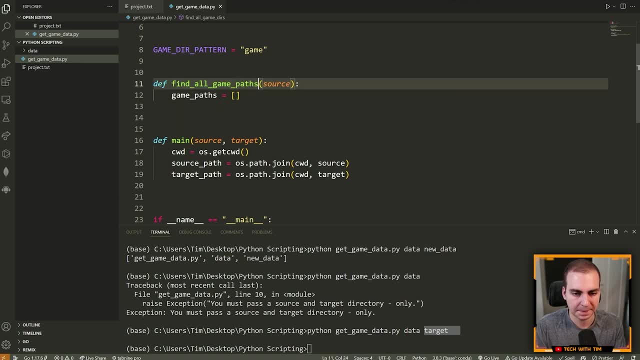 And actually I want to change this: say, find all game paths, because it's going to give us the full path, not just the directory name. Next, I'm going to say it for root: I believe this is going to be DERS files. 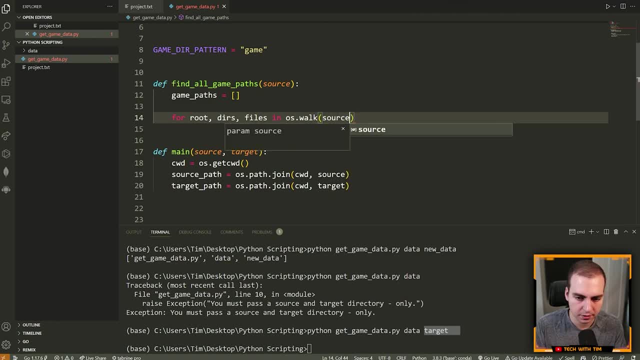 in os dot walk And I'm going to walk the source path. Okay, Now what walk will do is walk recursively through whatever the source directory is that you pass uh to this, this os dot walk command, So it's going to give you 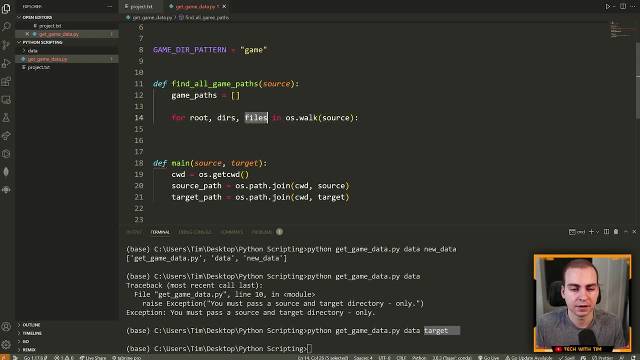 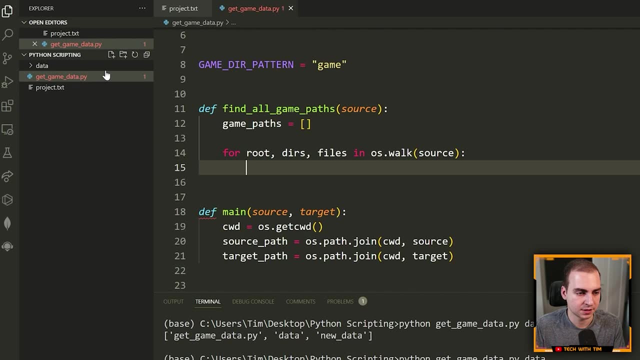 the root directory, the directories and the files that are contained in the current level that it's walking through. Now what this will do is recursively continue to look. So in this case it'll look in data, but then it would after. 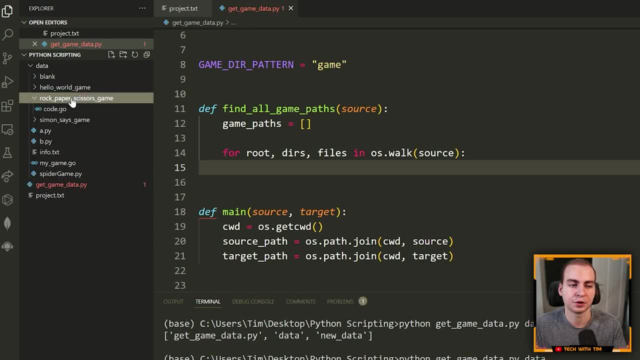 looking in data, look inside of blank, then look inside of hello world, then look at the inside of rock paper scissors game. It would look through all of those directories. Now, we only care about the directories that are immediately inside of data. However, if you 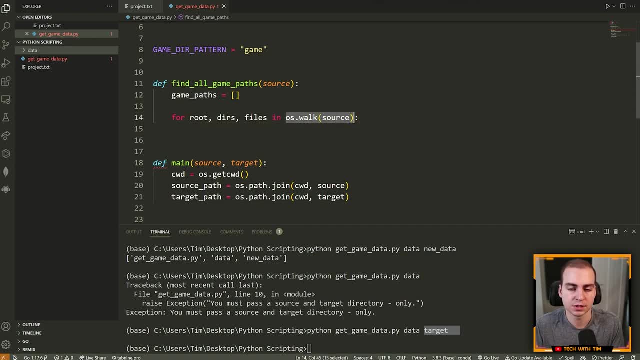 wanted to recursively look through all of them. this is what you would use, Hence why I'm showing it to you here Now, since we only care about the first kind of top level directory, we only really need to run this command one time. So 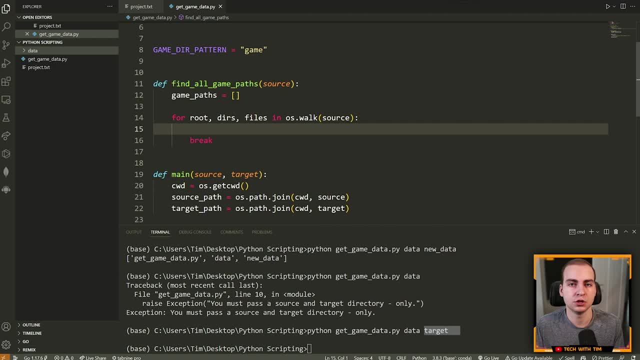 at the end of my four loop. I'm just going to put a break so that I only do this once, And this is just an easy way for me to grab kind of all of the values one time, right. So you just break at the end of the. 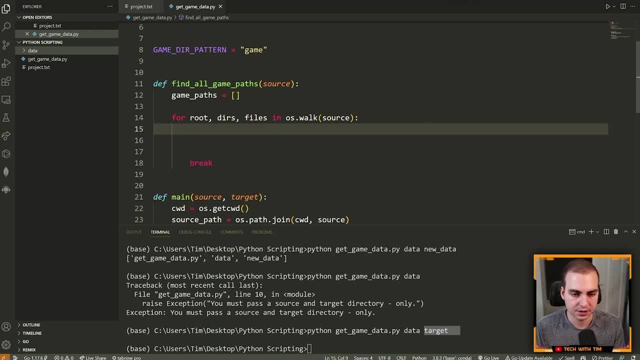 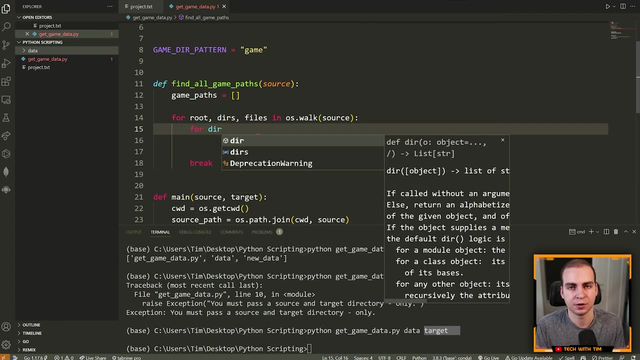 four loops. We only run this one time. Okay, Now that we've done this, uh, we need to loop through all of the directories. So I'm going to say for: and you should not use dirt, because that's a built-in command. So I'm 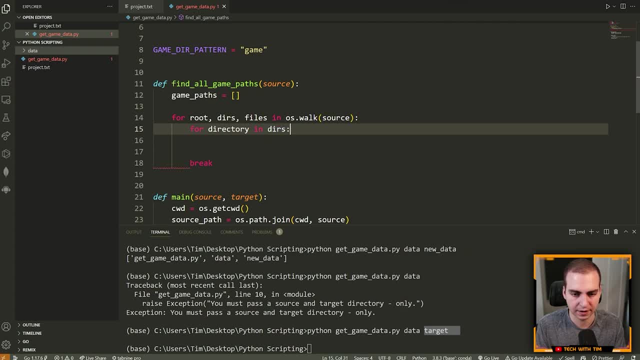 going to say directory in dirt, like that, And then I want to get the name of my directory and match that against my game dirt pattern. So what I will do is say if my game dirt pattern is in my directory dot lower and I'll put this: 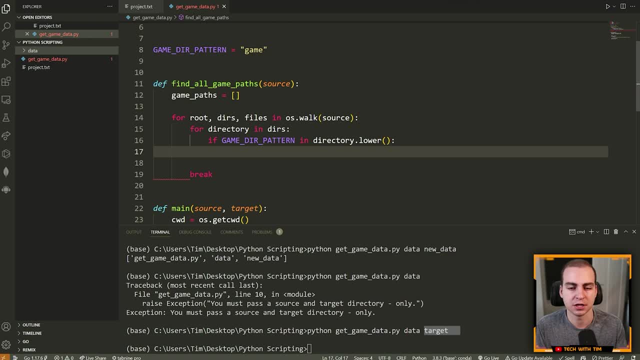 lower case, just in case we have a capital game or like a capital on the G or something like that. you don't have to do this, but I think it makes sense to do that. If this is the case that I'm going to add this path. 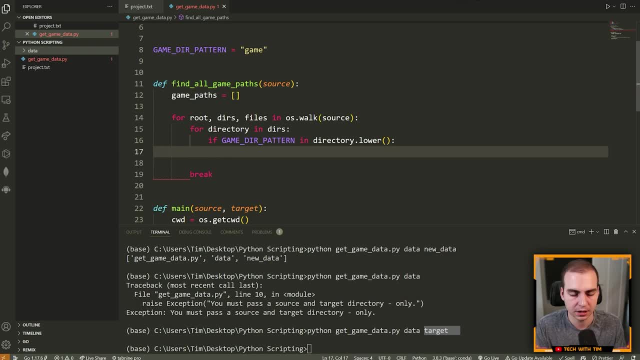 uh, to my game paths. So what I will do here is say my path is equal to os, dot path, dot, join. And then I'm going to take my source and I'm going to take my directory, like this, and I'm going to 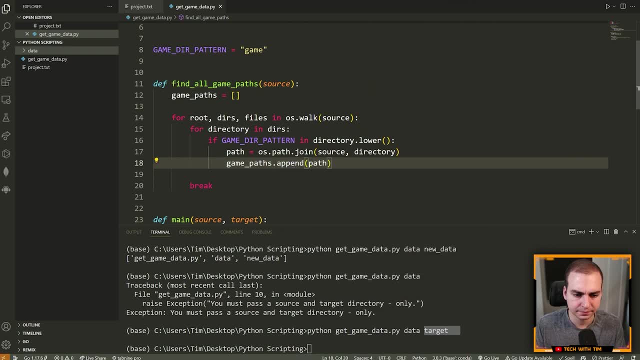 say game paths, Dot append my path. Okay, Then down here we will return our game paths. Now the reason I'm doing this is because this uh DERS list here gives me all of the names of directories, not the paths to those. 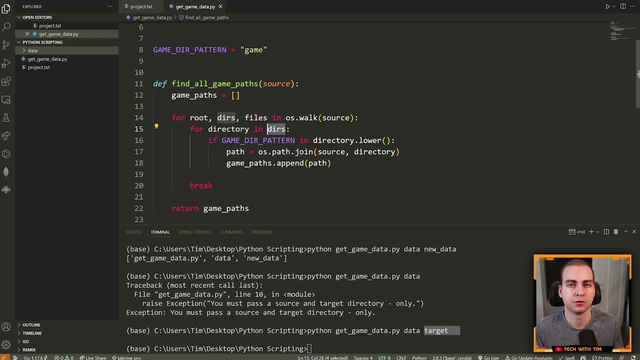 directories. Now here, I want the full path. The reason I want the full path is so that I can easily copy it later on. If I don't have the full path, I can still create that full path, but it's just easier to return all. 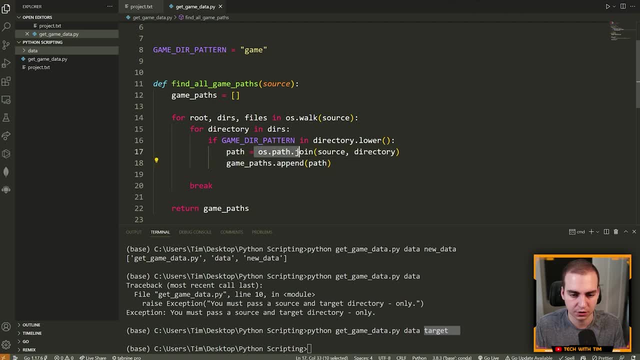 of the full paths right now. So that's why I'm doing it. So I'm saying path is equal to. oh, I stopped path dot join, taking my base path, where I know this directory is contained inside of, and then I'm joining them. 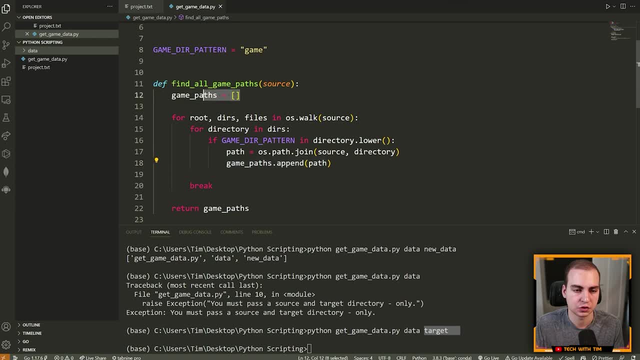 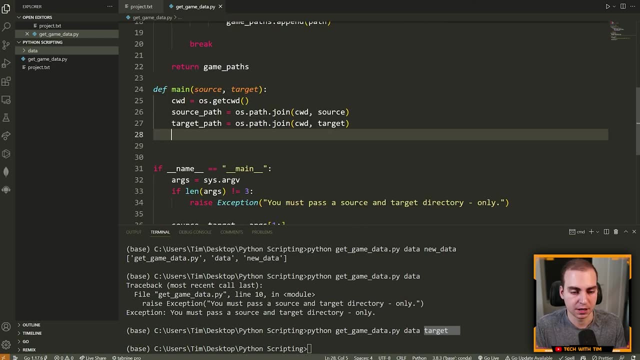 together, right, Taking the directory name, adding it to the base and then adding this to my array or list of paths, and then I will return that fantastic. So let's try this out now and make sure that this works. So let's say, our game. 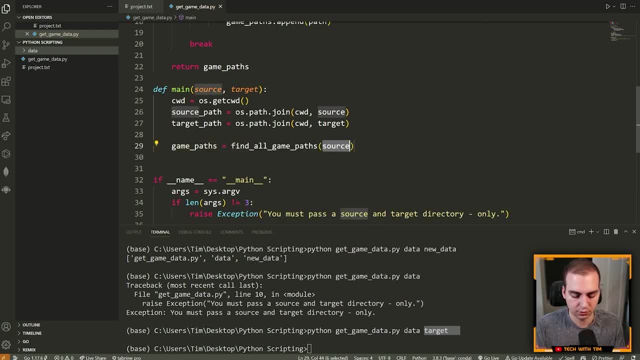 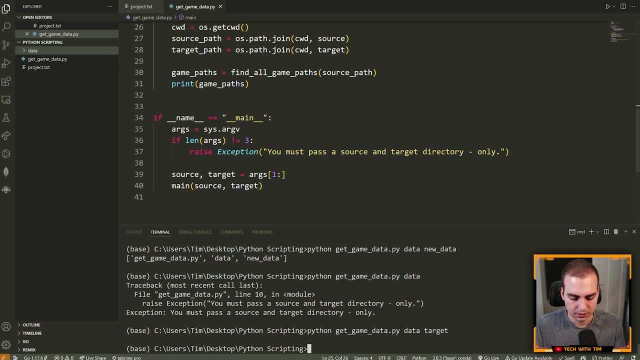 underscore. pass is equal to find all game paths, And then we'll pass here the source path. It will print our game pass, Okay, So let's give this a shot here and see if we had any errors or not. so here we're going to pass data, that's. 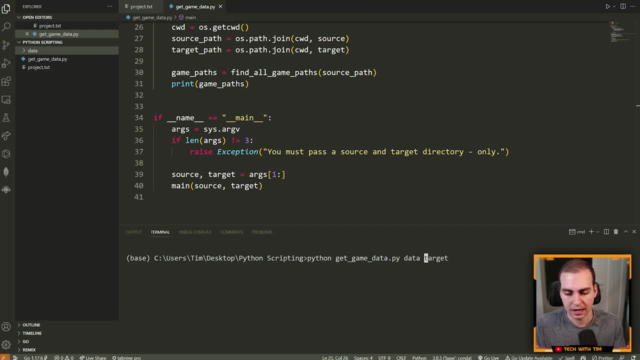 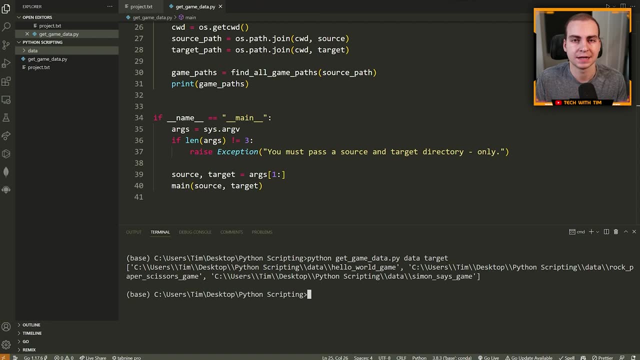 going to be our source directory, so make sure you have data there and then target will be our target, although it doesn't matter right now. all right. so notice now that i get my full paths to all of the directories that contain the name game. so i have my hello world, i have my rock paper scissors game. 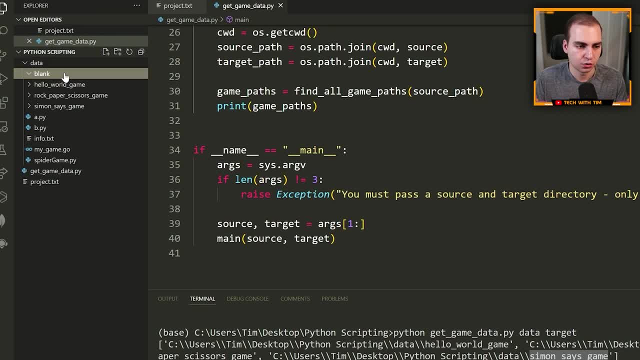 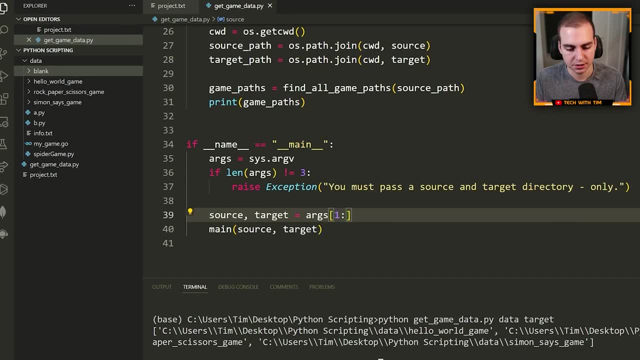 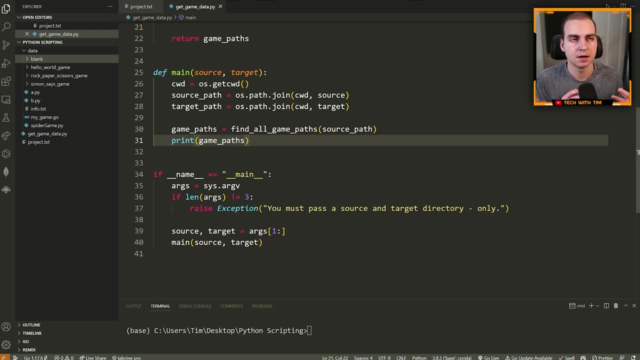 and i have my simon says game. now, notice that i've ignored the blank directory. i've ignored any files, even if my file had the name game inside of it, because i was only looking in directories. fantastic, okay, so that is working. the next thing that i want to do here is i want to take all of 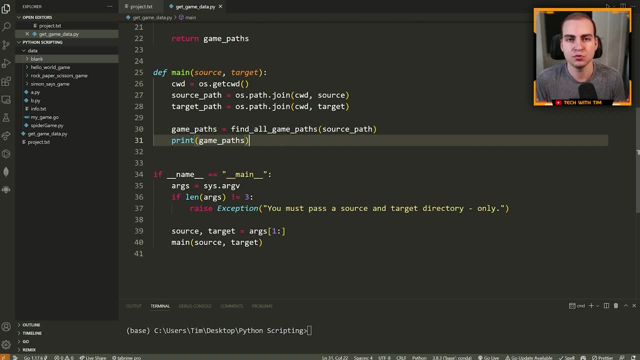 these paths and i essentially want to just get the new directory name that i want to copy these directories to. i know this seems a bit weird, but remember, what we're doing here is we're taking all of these directories and we're copying them into a new directory, but we're removing the 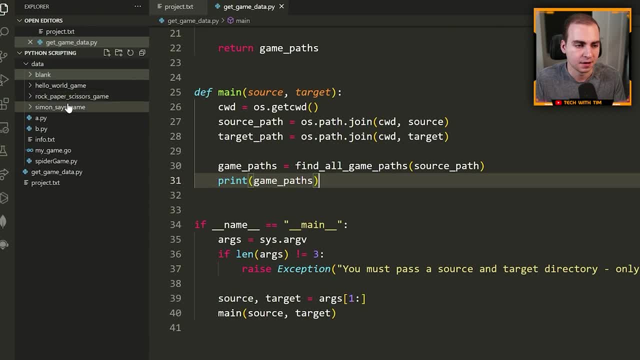 game, game directory and we're copying them into a new directory but we're removing the game game part from that directory name. so when i copy, you know simon says game. i'm just going to copy simon says not the game part into a new directory. so i need to get that kind of destination path before. 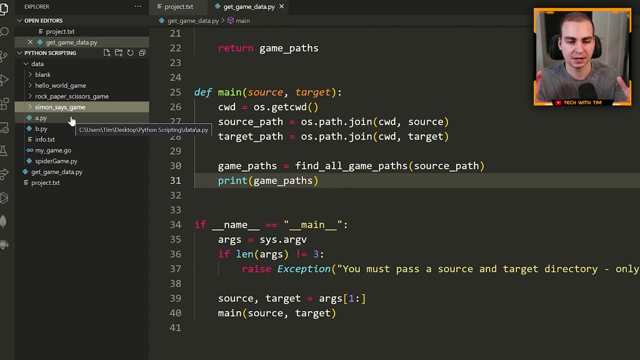 i can perform that copy, because to do a copy, i need a source, i need a destination. right now we just have the source, so we have to create the destination, and one thing we also have to do is create the new directory, and we can actually create the new directory right now. so let's. 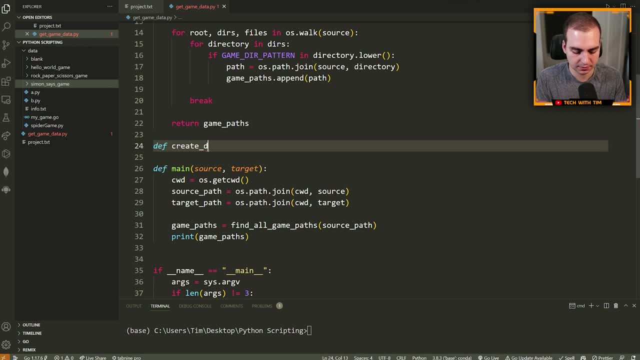 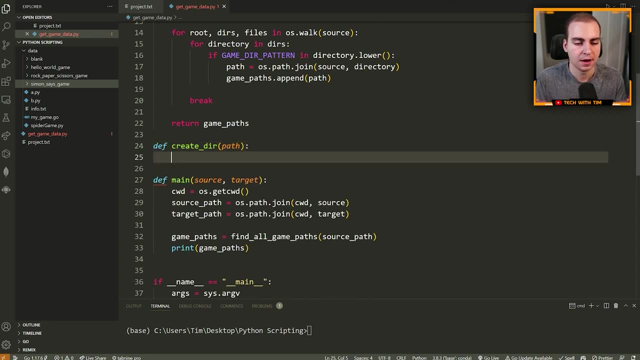 make a new um function here and say create underscore, underscore, dir, and all we'll take for this is the path to the directory that we want to create inside of here. i'm first going to check if this directory exists. if it exists, i don't need to. 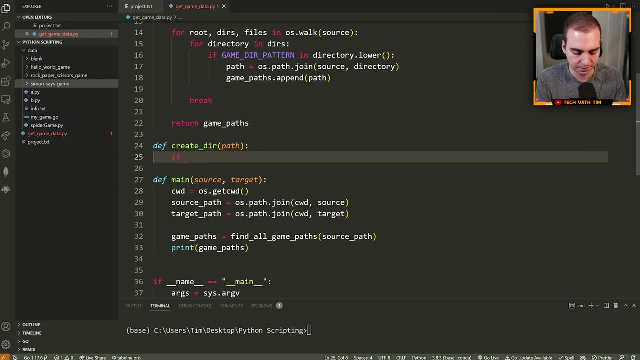 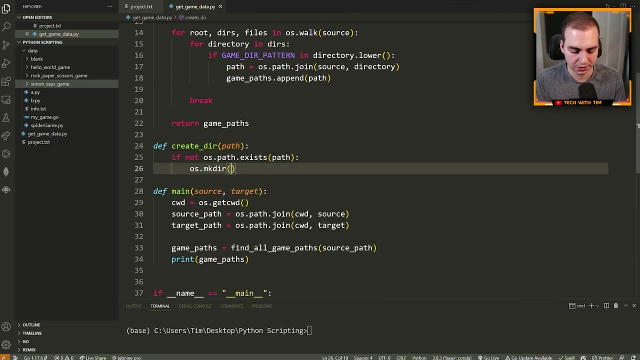 create it. if it doesn't exist, then i will create it. so i'm going to say: if not, and then this is os dot. uh, actually, is this going to be? i think it's ospathexists. yes, okay, that's correct. so if this does not exist, then i will say osmkdir, which stands for make directory, and i will make the. 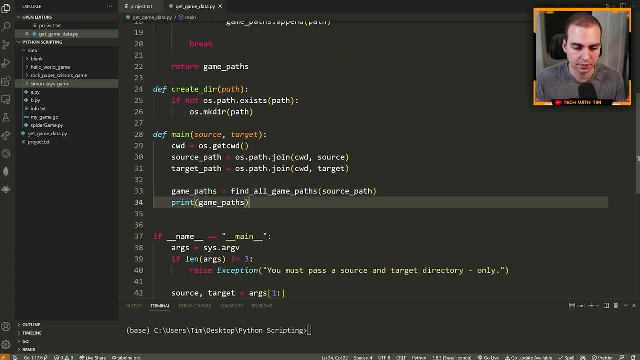 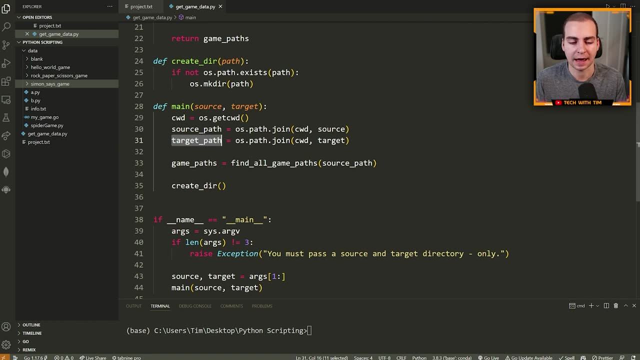 directory at this path. okay, that's it for creating the directory. so let's go here and let's say create dir and the directory that we want to create is going to be the target path, right, so we'll just pass the target paths path there. sorry, okay. next we want to get all of those destination paths, so 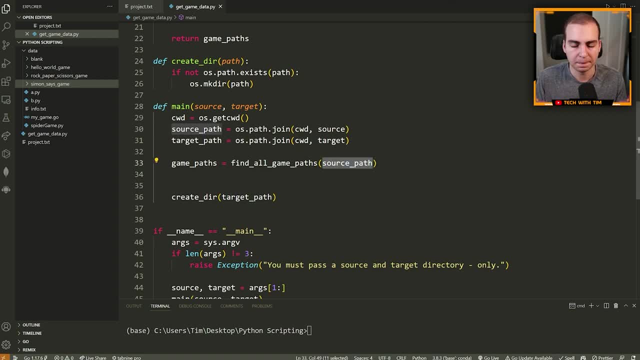 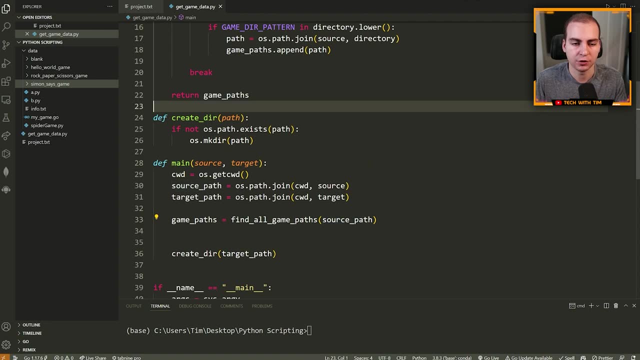 i need to make a function that is essentially going to look at this whole path and it's just going to give me the directory name, uh, but removing the game aspect. now, i know this seems a little awkward, so i'm doing it. i'm doing it intentionally, so that i can show you how you. 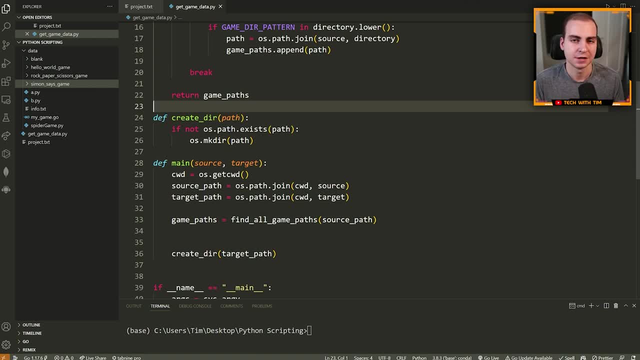 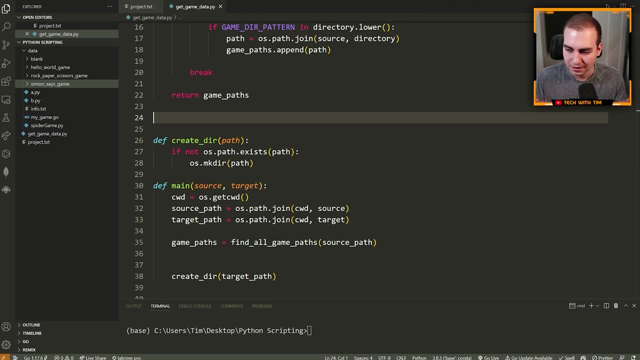 strip apart paths and take like certain components of the path. so, believe me, i know there is an easier way to do this, but i'm trying to show you like how you can use a lot of different commands here, so hopefully you appreciate it. anyways, let me just quickly look at my cheat sheet here. okay, 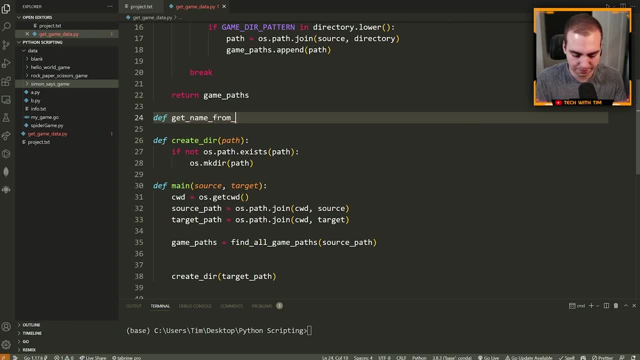 uh, and i'm going to say that this is called get name from pass. i'm going to take in my paths and i'm going to take in what i want to strip off of my directory name. so i'll call that to strip. i don't really know what else we would call that. okay, so i'm going to go here and say new names. 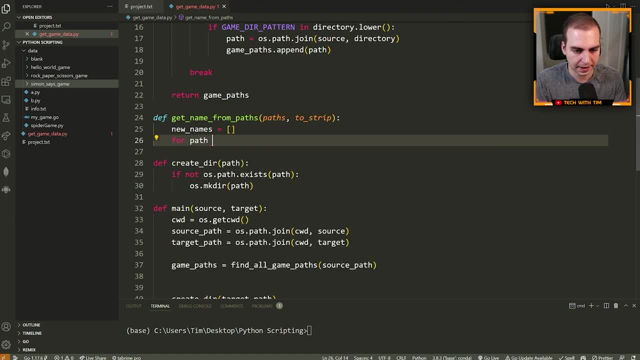 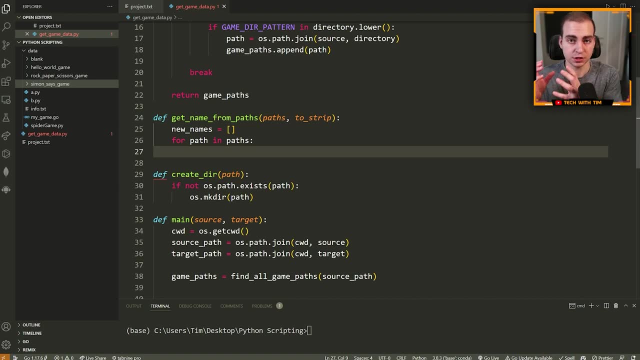 is equal to an array and i'm going to say for path in paths. now what i want to do is i want to split my path into the just the directory and the base part, right, so like the parent directory, of just the directory because, remember, we have the full entire path. so when we had game pass, we have the. 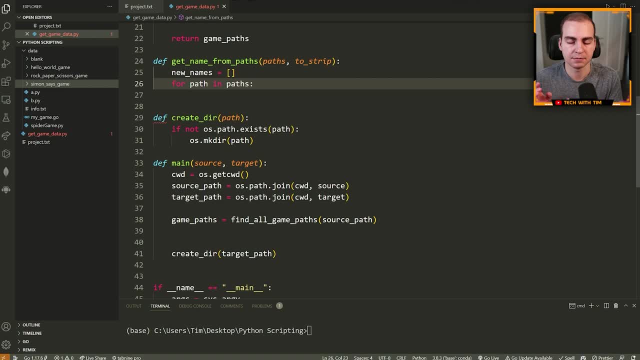 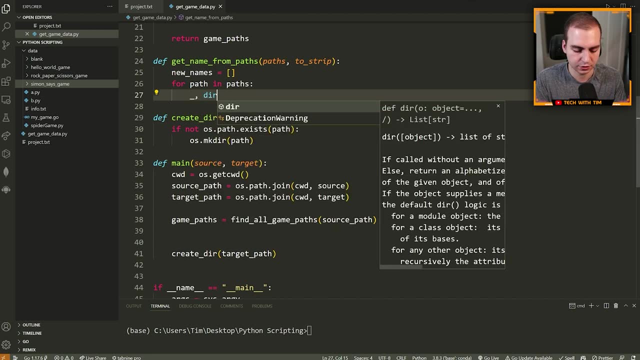 entire path to the game directory. so we're going to split it to just the game directory and then base path is now the way we do. that is, we can say underscore, because we don't care about the beginning part, and then we can say dir. underscore. name is equal to os, dot, path, dot split, and then 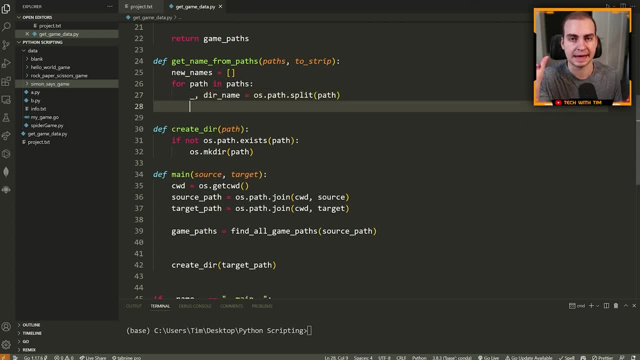 we can just split the path now. this is automatically just going to give you the very last aspect of the path, whether it's a directory or a file or whatever it is- and then the remaining part of the path on the left side. again, don't try to get clever and do this yourself by splitting different, uh like. 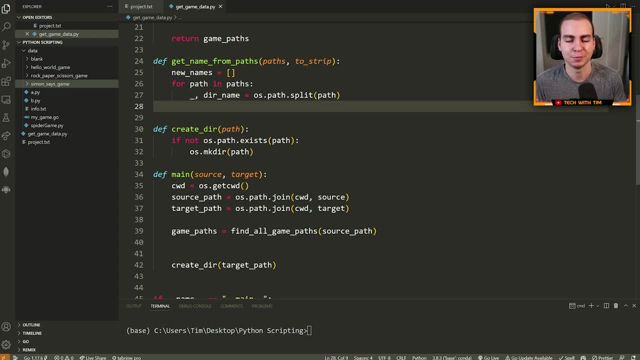 slashes or trying to find the path divider. just use these built-in functions, because they handle the different operating systems for you. okay, so now we have the dir name. now what we need to do is remove the game aspect or whatever aspect from this dirty. so i will say: new dir name is equal to my dir name, dot replace. 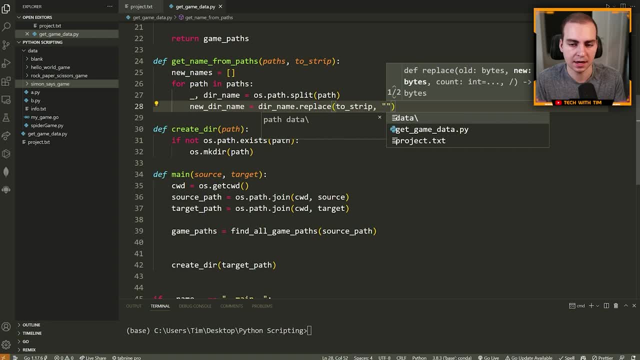 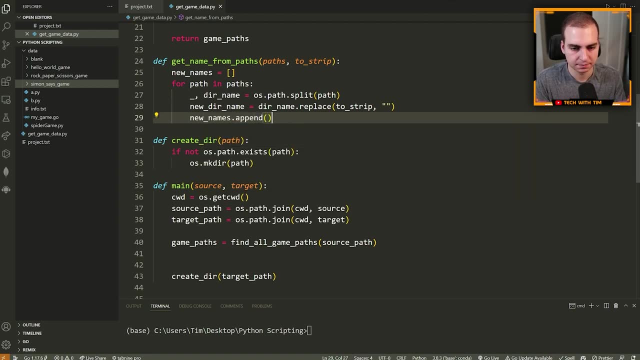 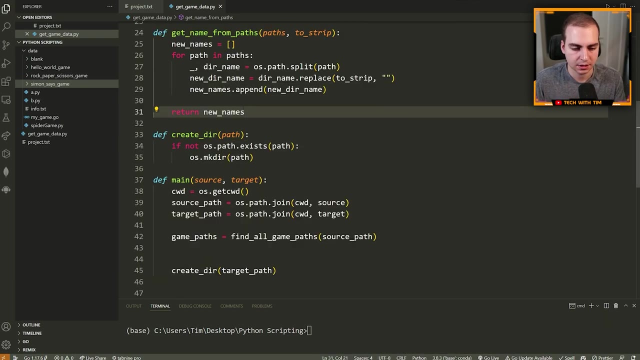 and i'll replace whatever the two strip string is that we pass, which will be game, with an empty string, which will just get rid of it from the uh the directory. then i'll say new names, dot, append my new dir name. then i will return my new names. fantastic, okay. so now let's get our new names. so let's say new. 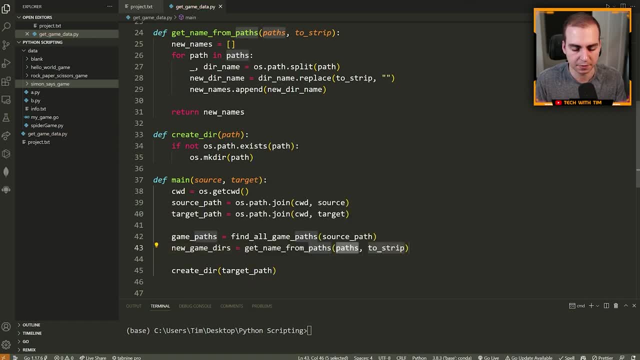 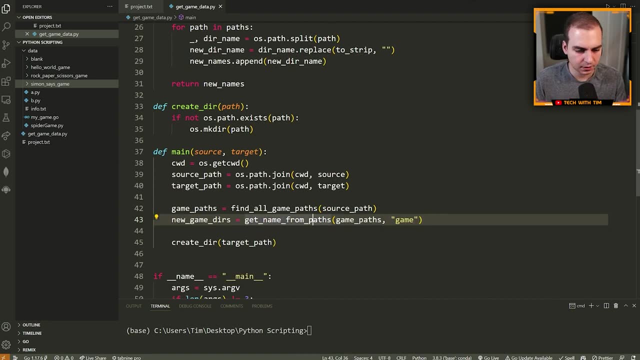 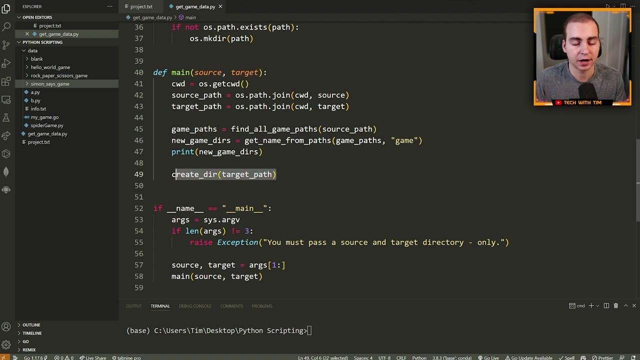 game dirs is equal to get name from paths, and our paths are going to be the game paths- and to strip- we're just going to strip off the string game. fantastic, now let's print our new game dirs. all right. now notice, i've create directory as well, so we should see that a new directory gets created. 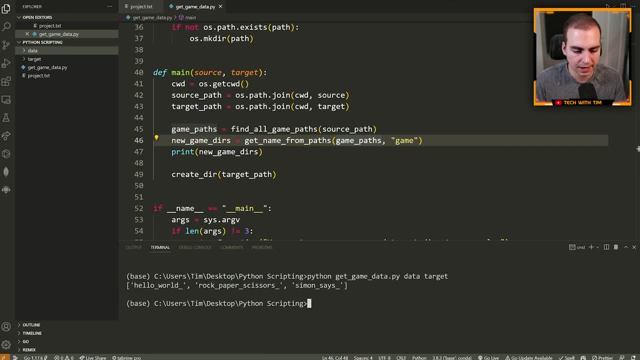 here when i run this. let's try it and see what we get and notice. now that we get hello world rock paper scissors, simon says plus the target directory was created, so i'll delete that so we can create again later. okay, now we do have the underscore here. now that makes sense, right, because we're just looking for. 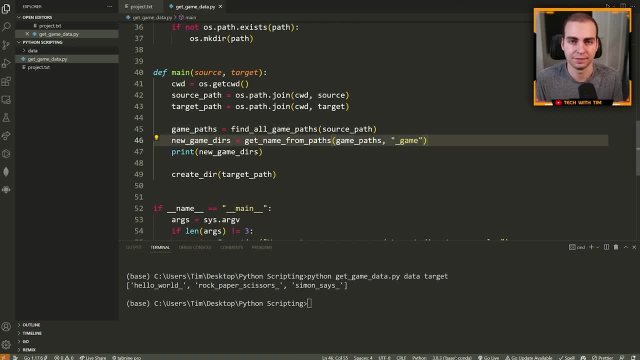 game. now, in this case we can look for underscore game and we can remove that entire thing, but it's up to you how you want to do this right. if you look for underscore game, then if you started the directory name with just game, it wouldn't count or wouldn't remove it, so you could do some advanced logic to remove this if. 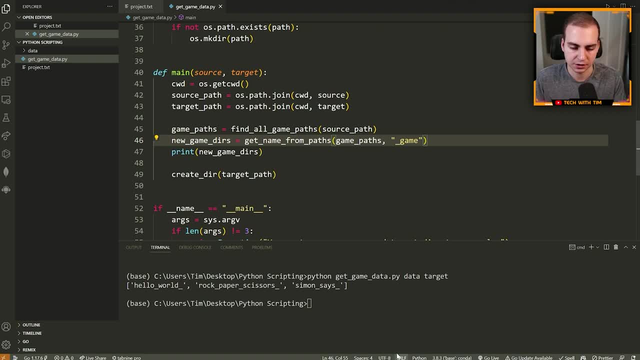 you want, but, But for now we'll just make it underscore game. I think you guys know what I'm saying here. OK, so let's clear that. And what do we need to do next? Well, now that we have our kind of destination, 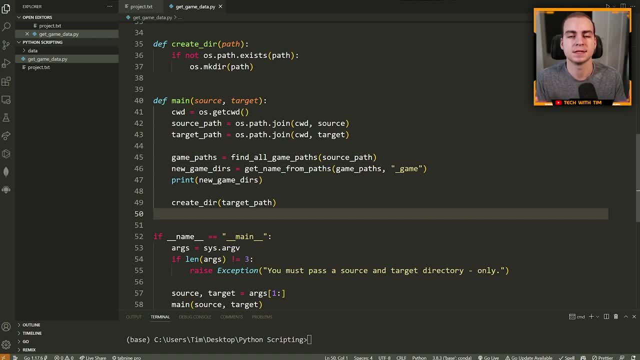 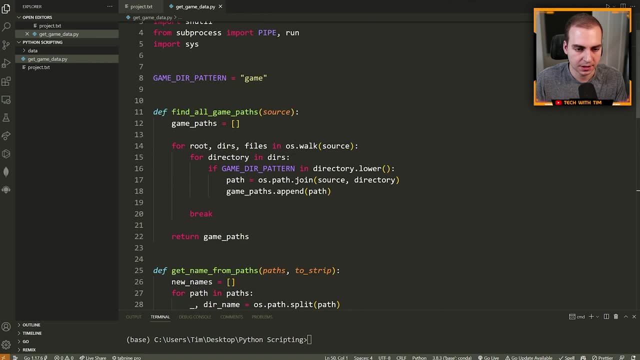 our source directories for all the games, as well as where we want to put these games. Now we need to well need to write them right, Like we need to actually do the copy operation. So what I'm going to do is make a new directory. 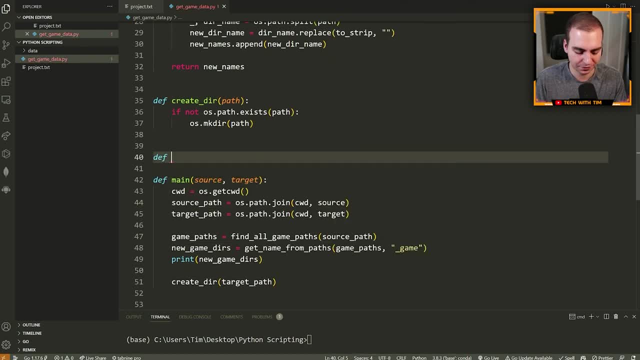 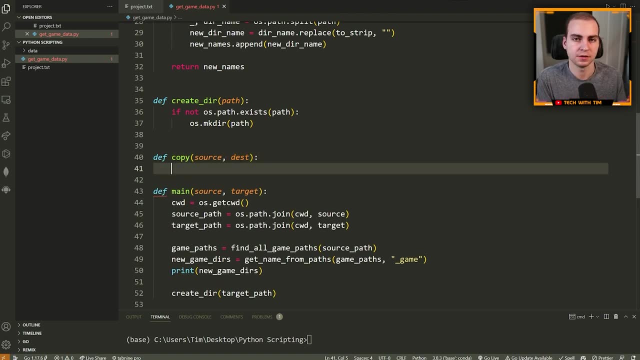 or new function, not directory, And I'm going to call this copy OK. now what copy is going to do is take a source and a destination and it's going to copy the source into the destination. Now I will actually kind of change this a little bit. 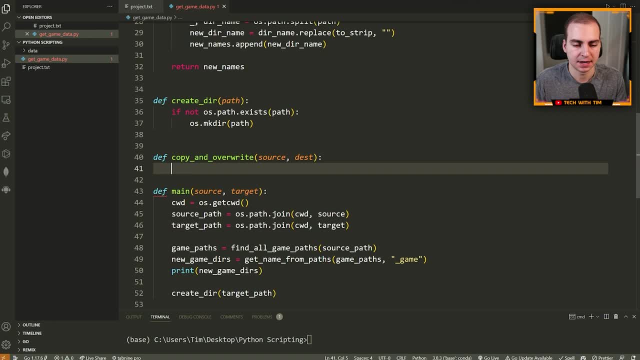 And I will say: copy and overwrite. Now, the reason for this is that if the directory already exists, I want to overwrite it, And I will show you how we can do that. Now, keep in mind the commands I'm going to use here. 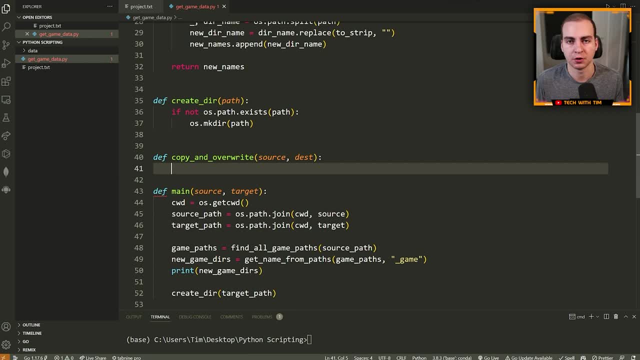 are just one option to do this. There's like a million ways you can go about copying and deleting directories, But I'm going to show you how we delete a directory if it already exists And then, of course, how we copy it. 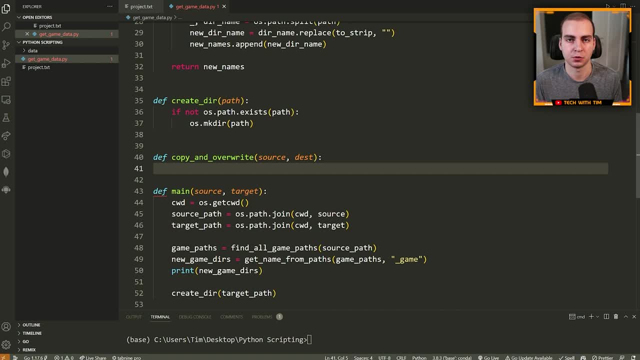 And this will be a recursive copy which will copy everything. So if there was another directory inside it would copy that directory as well in all of the contents of that directory. A lot of the copy operations don't do that, So just keep in mind. 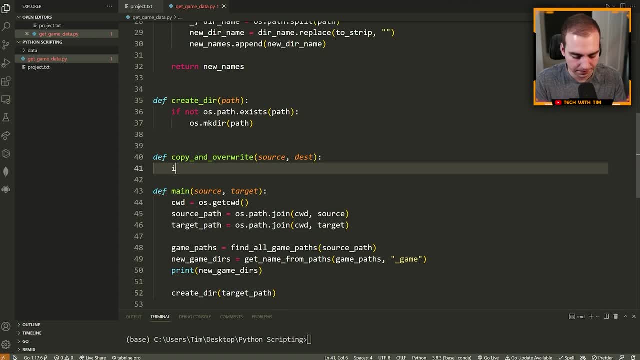 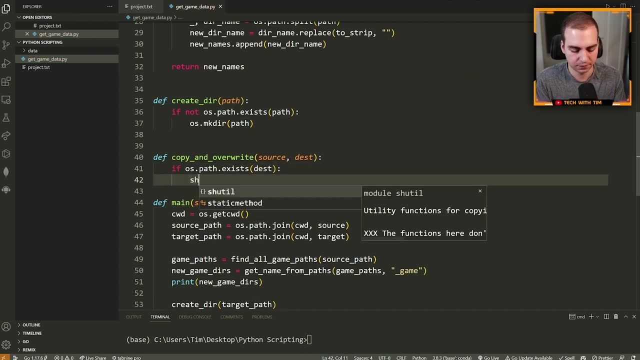 if you want a recursive copy, you probably want to use the option I'm showing you here. So I'm going to say, if OS dot, path dot exists, destination, that I need to start by removing the destination folder which I'm going to use my SHU till four. 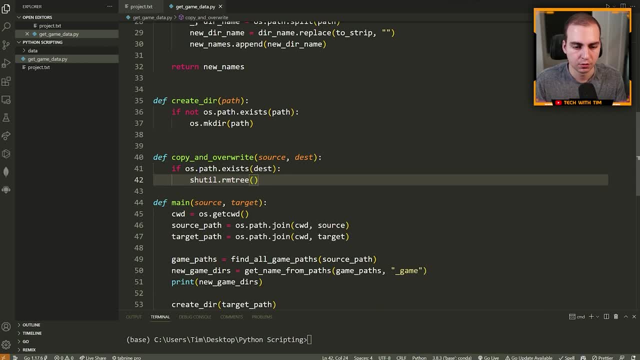 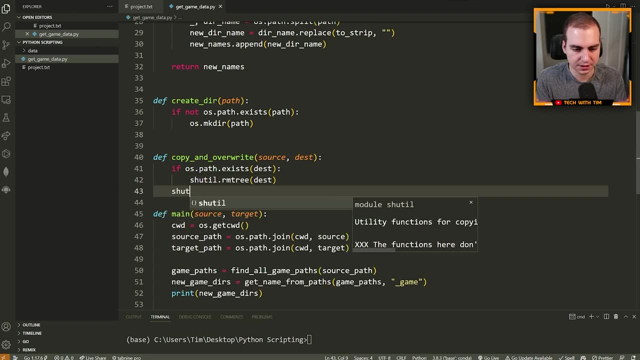 So I'm going to say SHU till dot RM tree, which stands for remove tree, which is essentially a recursive delete, And this is going to be the destination Now. after this, I'll say SHU till dot copy tree, And then I will copy. 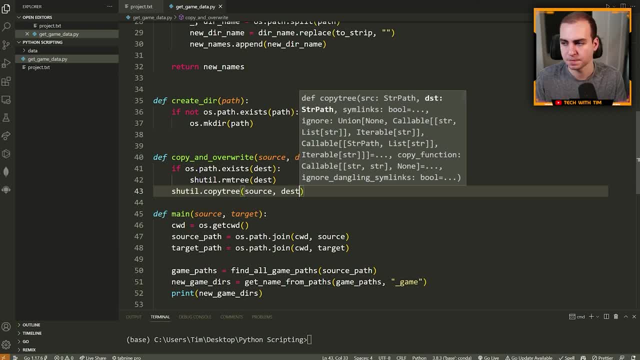 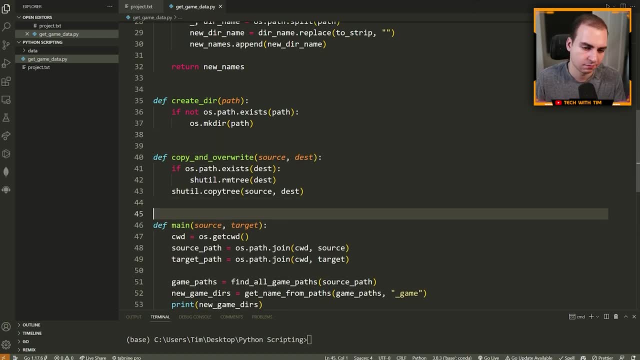 the source to the destination. All right, That's all good. That's all we need for copying and overriding, Or overriding however you want to. I think overwrite is the correct term. OK, so now that we've done that, we can use this function. 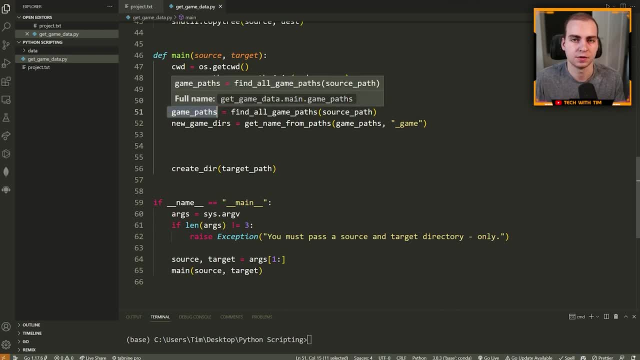 So we need to essentially loop through all of the different paths that we have, So the source paths as well as the destination paths, and then we need to run this copy command, So I'm going to say four, and we'll call this SRC destination in. 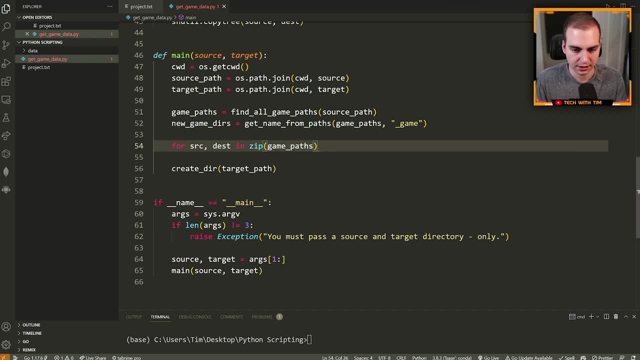 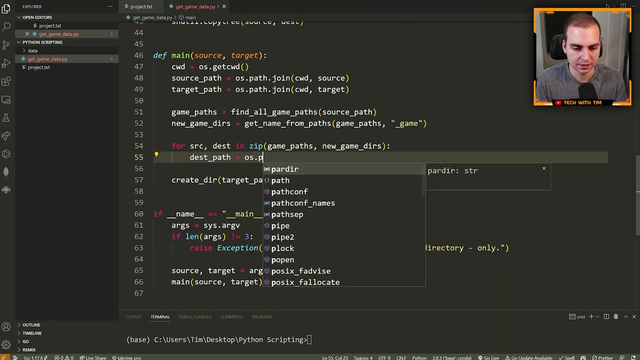 I'm going to use this zip function. I'll explain how this works in one second, but I'm going to pass my game paths and my new game directories. I'm going to start by saying: my destination path is equal to OS, dot path, dot. join. 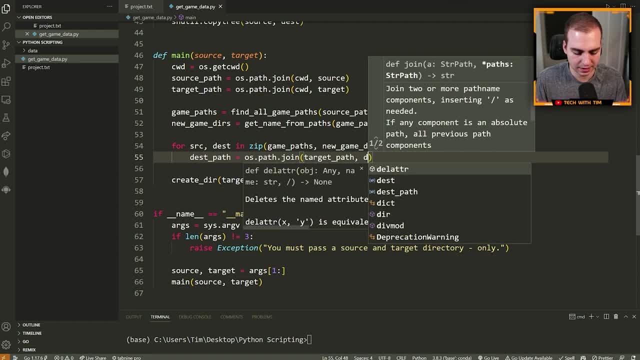 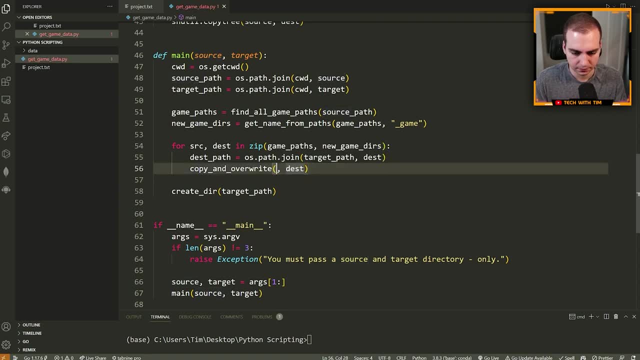 And I'm going to join my target path with my destination folder name. Then I will run the copy and overwrite function with my SRC and my destination. OK, so let me explain how Zip works. What Zip will do is it will take matching elements from two arrays. 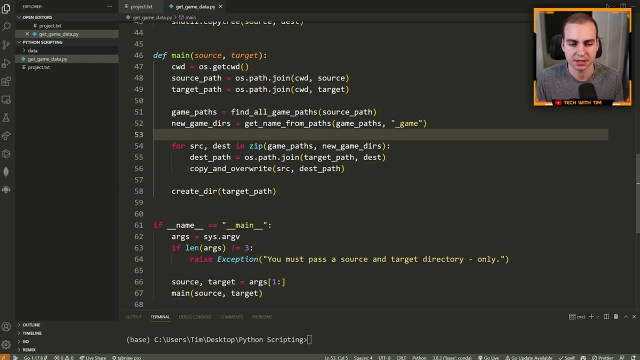 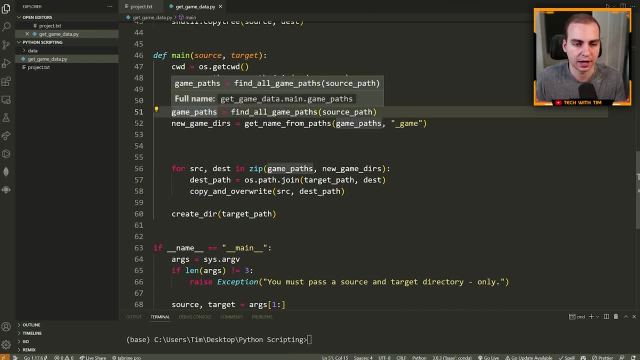 and combine them into a tuple, which then gives me access to them at the same time. So notice, right, these arrays, or these lists, are going to be the same length. So this first one is going to be all of the original game paths. 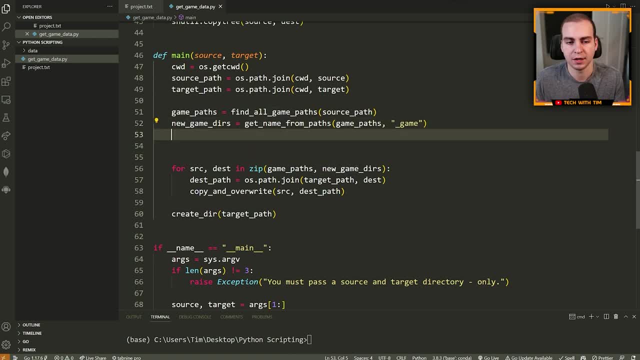 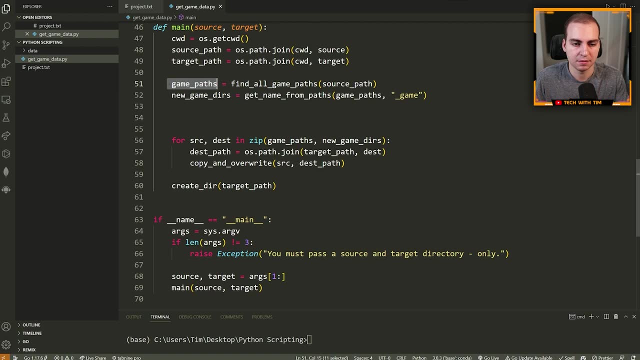 and this is going to be our new game directory names that have this underscore game removed. Now I want to be getting the game path associated with the new game directory name because I want to copy whatever is here into this new directory name. So I zip them together. 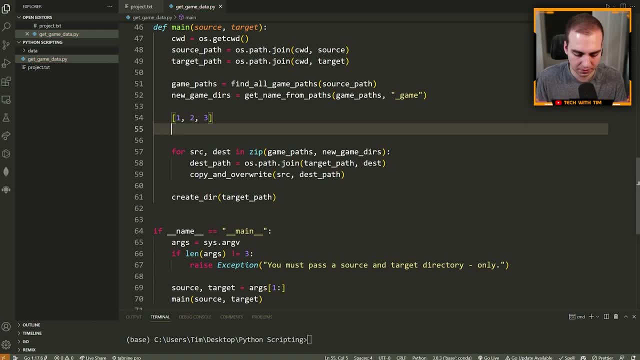 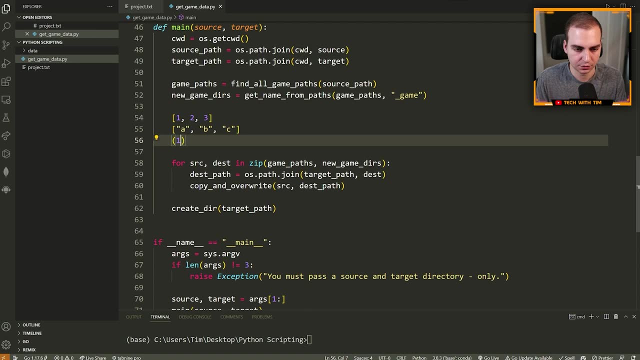 So, to show you a quick example, if we have 123 and we have like a, B, C, then if you zip these together, what you're going to get is an array that has one and a, or a tuple story that has one and a. 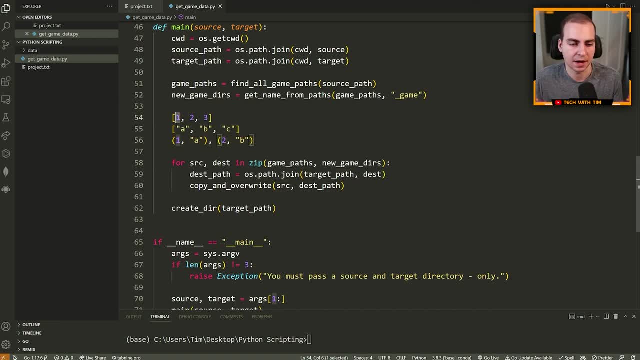 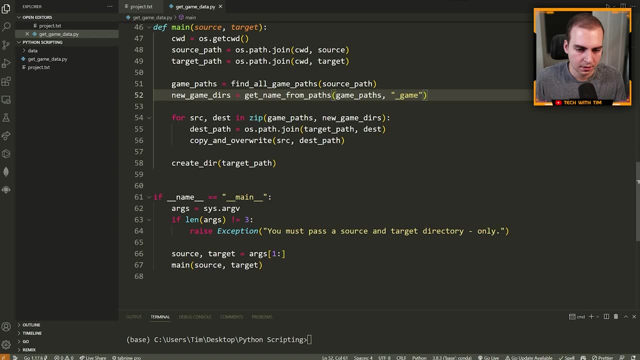 two and B et cetera, just combines them together. So the matching elements at their indices get kind of matched up, And that's why I can say source, destination here and iterate through the zip. OK, so now this should actually be good. 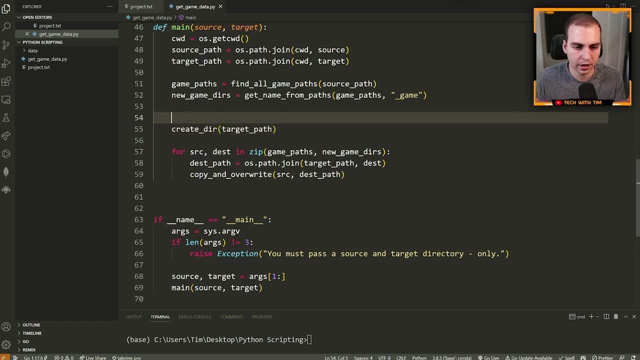 However, I need to make sure that I create this directory before I do this, Otherwise we're going to get an error where it's our path doesn't exist. OK, so let me slow down for one sec. I'll explain what we've done. 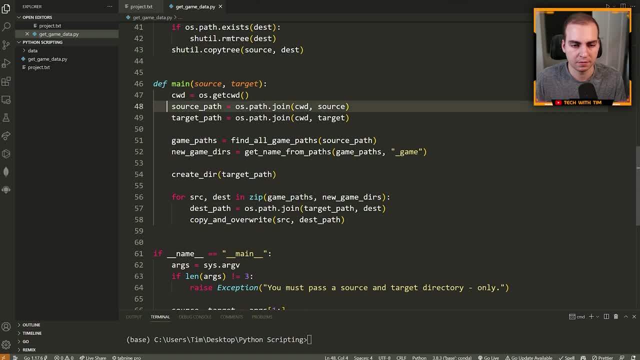 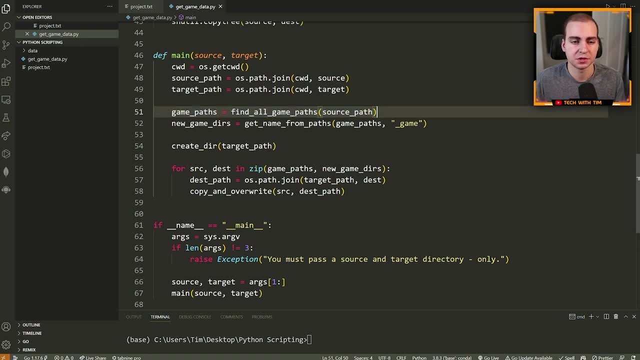 We can run it and we can continue. So what we've done here right is we've gotten the source path as well as the directory path. We have found all of the game paths that we're interested in, So essentially those directories. 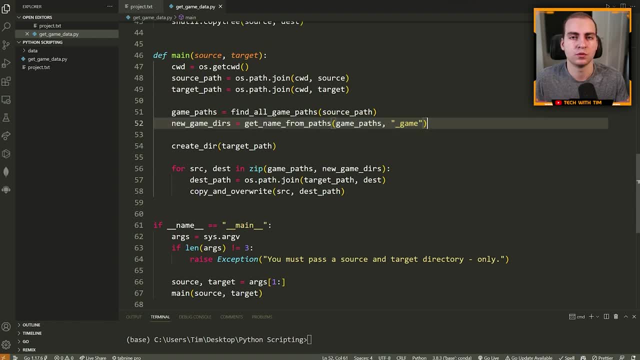 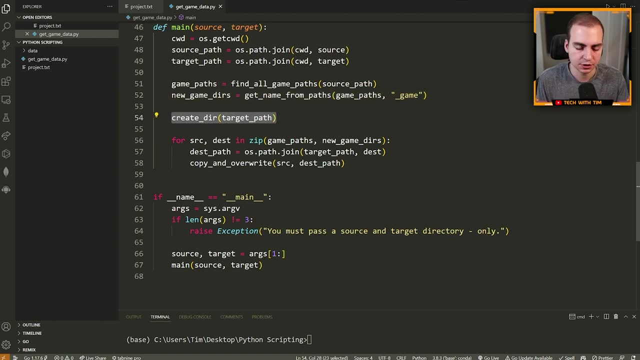 from the source directory. we have then found what we want our new game directory names to be. We have then created the target directory where we want to copy all of these into, And now we are actually performing that copy operation. OK, so we're at that point. 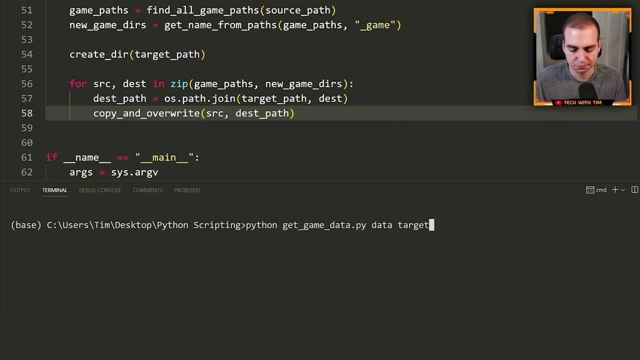 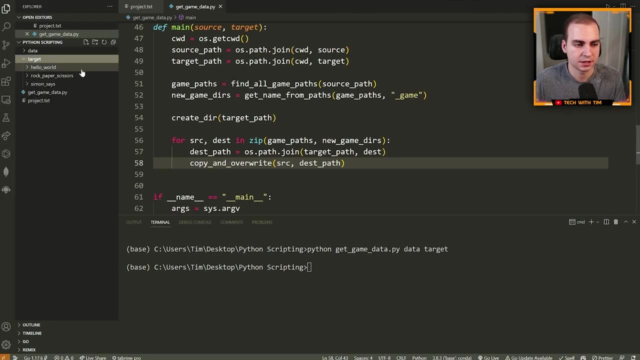 So let's run this and see how it works. So Python get game data and then we're passing data and target. I hit enter And when I look in target here you can see I now have Hello, World, Rock Paper, Scissors and Simon. 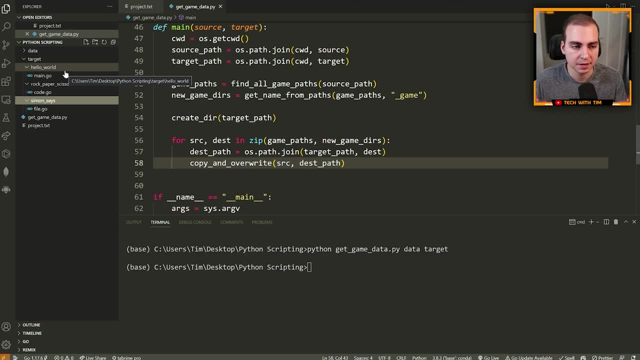 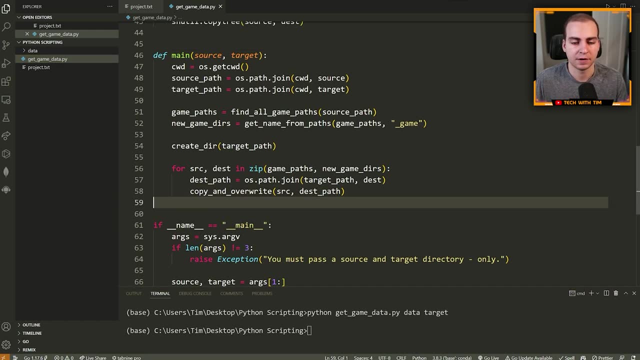 says With the contents of those directories, because I just copied them in Perfect, So now let me delete this and we can continue. So the next thing I want to do is write a JSON file that just has some metadata about the different games. 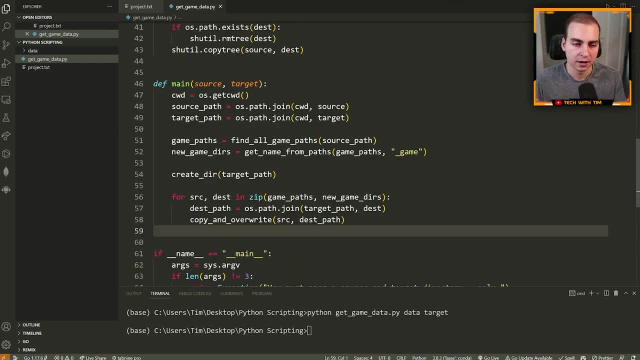 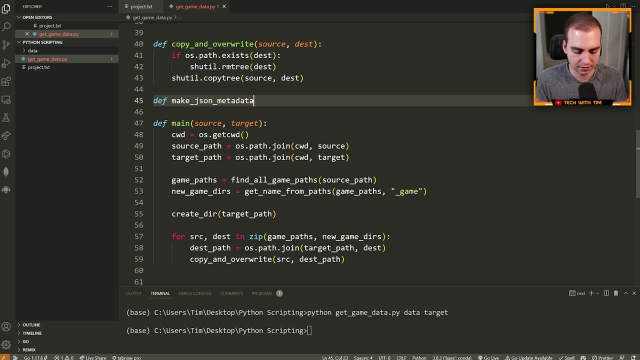 So what the game directory names are and how many of them there are. This is fairly straightforward. So let me create a function. I'll say make JSON meta data file, And here I will just take my path. So what do I want the file to be? 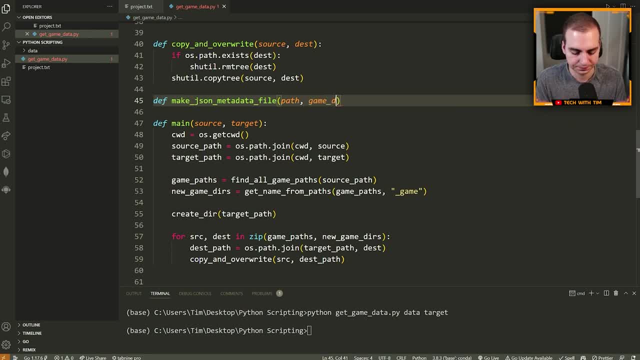 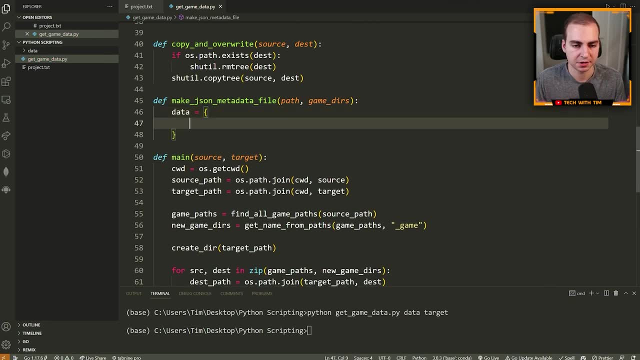 or where do I want it? I want it to be, And then I will take my game Ders. OK, now, here I'm going to say that my data- this is the data I want to write into the JSON file- is going to be equal to: 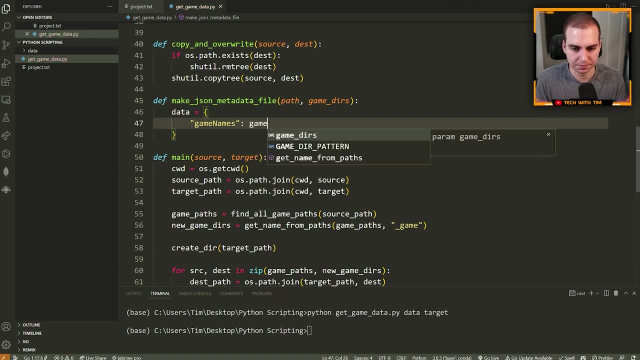 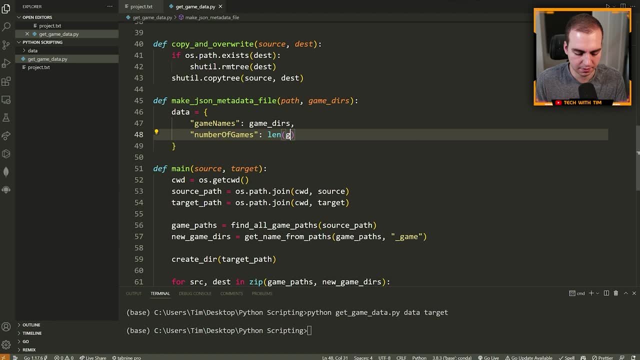 I will say my game names is simply my game directories, And I will say number of games And this will be the land of my game. Very straightforward, Not the most useful data, but just want to show you how we write JSON. So now there's a. 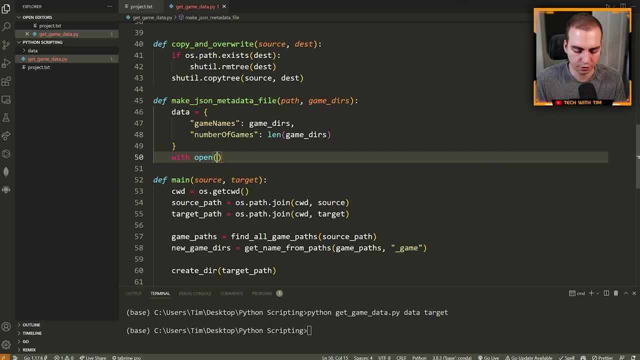 few ways to do this, but the preferred method is to do the following. I'm going to say with open path in W mode- W stands for right. This will override the file if it already exists. If you wanted to read the file, 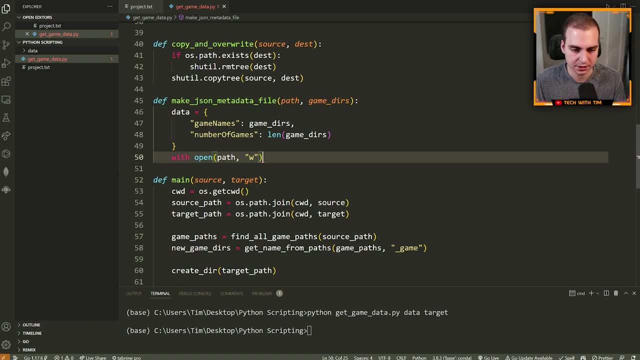 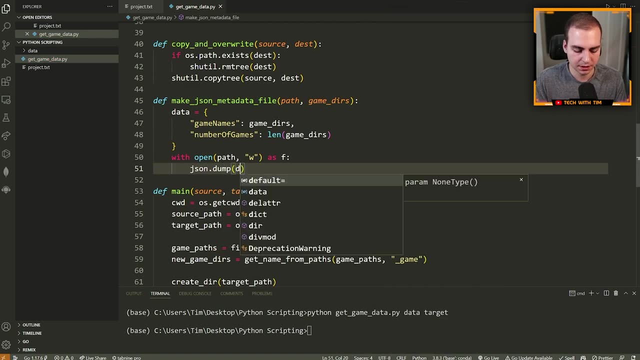 you'd use R, So I want to write and override: if it exists. I'm using W and I'm going to say as F, and then I'm going to say JSON dot dump and I'm going to dump my data into my file. Now, if you've ever seen 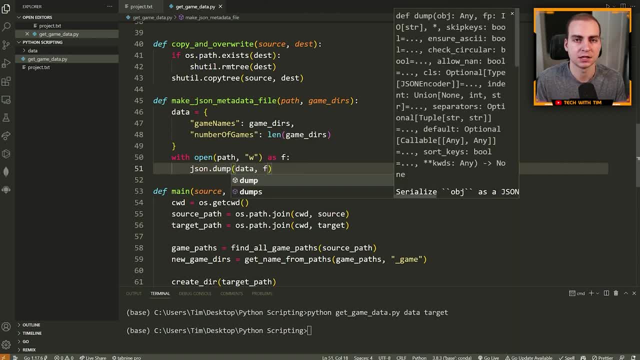 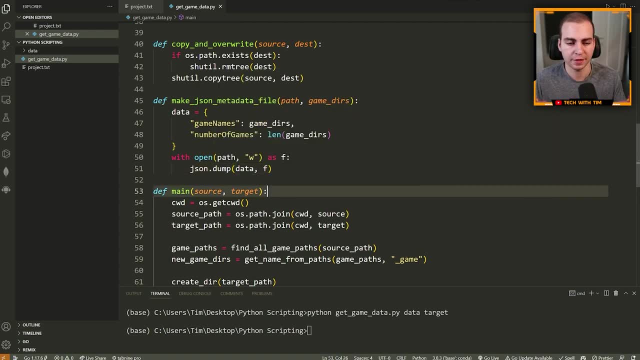 JSON be used before with dump s. dump s stands for dump string and that's going to dump the JSON data you have into a string. We don't want that. We want to dump it into a file or just really save it into a file. 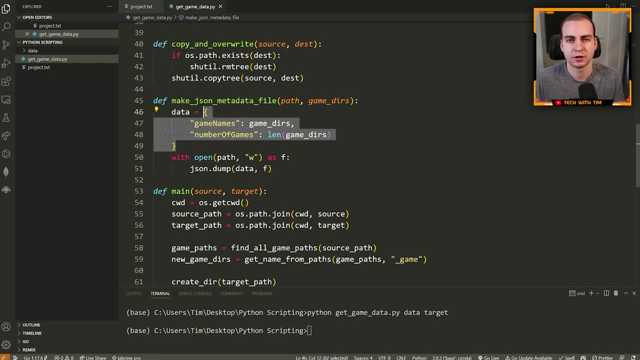 So we pass the data that we want to save, which in this case is a Python dictionary, which can kind of be represented as a JSON object, And we want to save it into this file object that I'm opening using something known as a context manager. 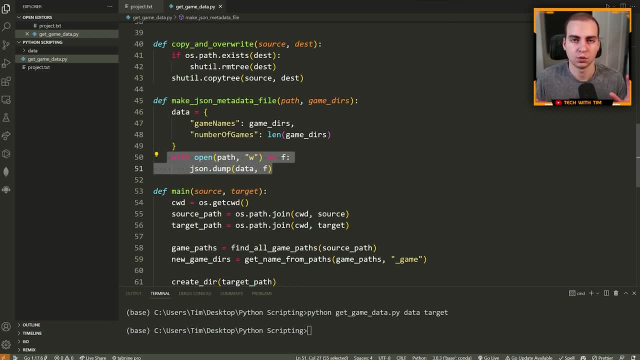 Now, the reason I use this is because as soon as we're outside of this with, we are automatically going to have the file a closed for us. If we didn't use with, we would have to manually close the file and there can be some problems. 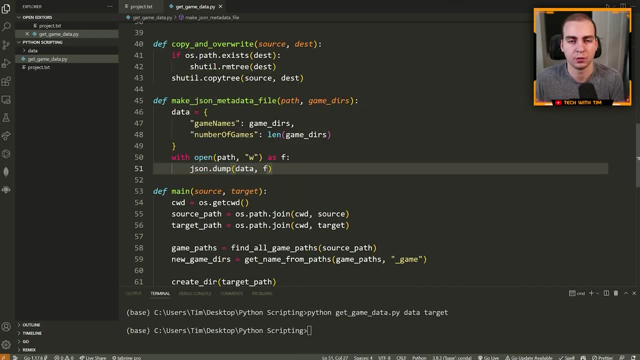 doing that, especially if an error occurs before we're able to close the file, we can have kind of a memory leak going on. So it's just preferred to use this, referred to as a context manager, that just make sure your cleanup operations happen, no matter what. essentially, 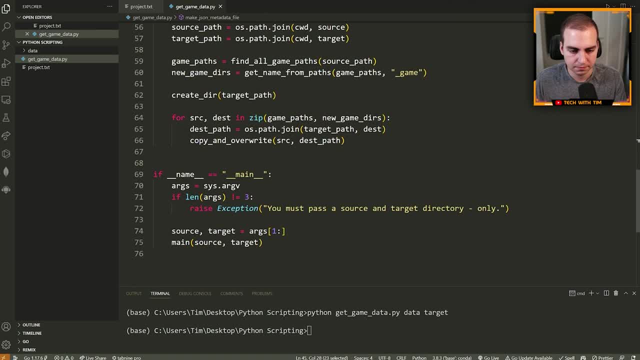 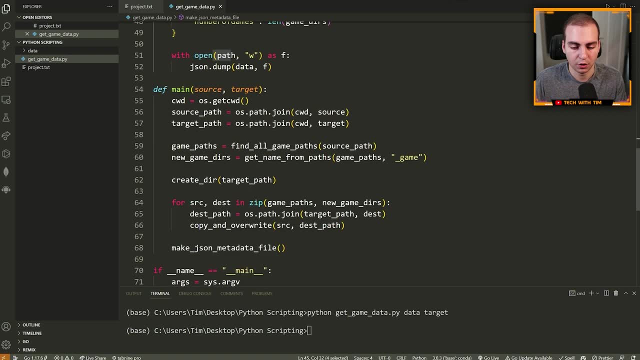 OK, so we have this JSON metadata file, So let me copy this function. Let's paste it here. We'll say: make JSON metadata file And now we need to pass a path that we want to use. So I'll say JSON underscore path. 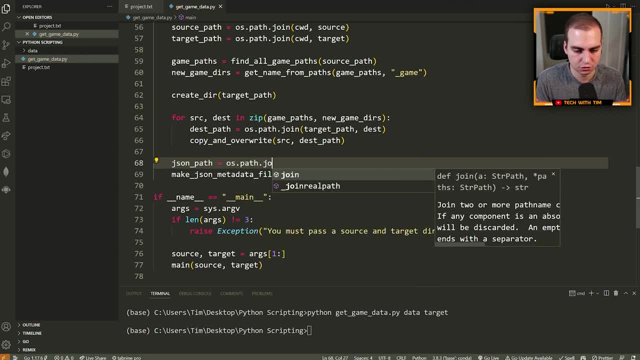 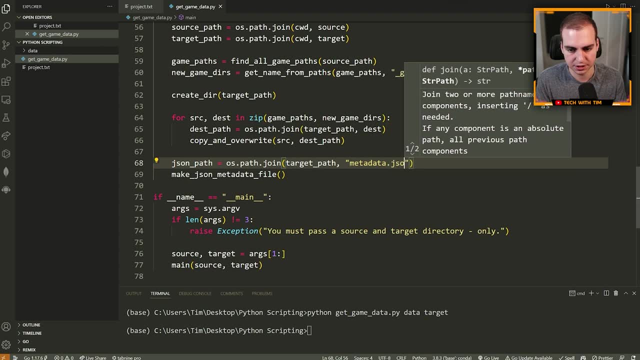 is equal to OS dot path, dot join, And I will join my target path with my metadata dot JSON name. So I've just come up with this name. You can name it anything you want, And then I will pass here the JSON path and my new game. 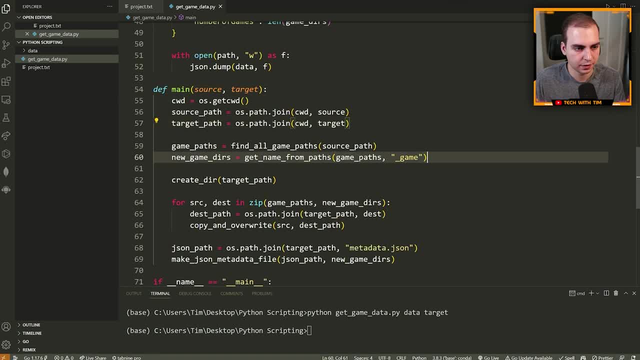 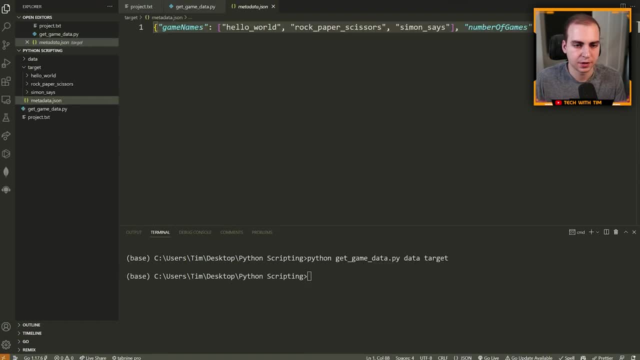 There's right, There we go OK. so let's run this again and see if it creates the JSON file. OK, go to target and notice we now have our JSON file. If I save it, we'll auto format here and you can see. 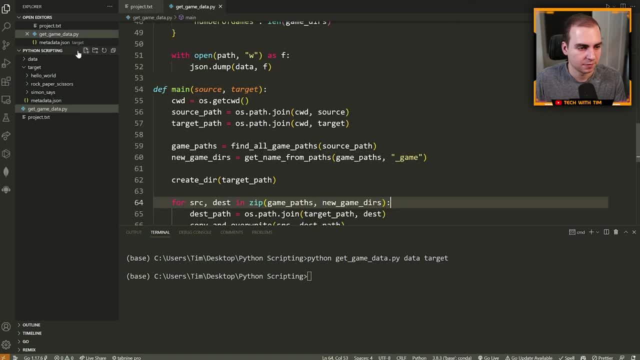 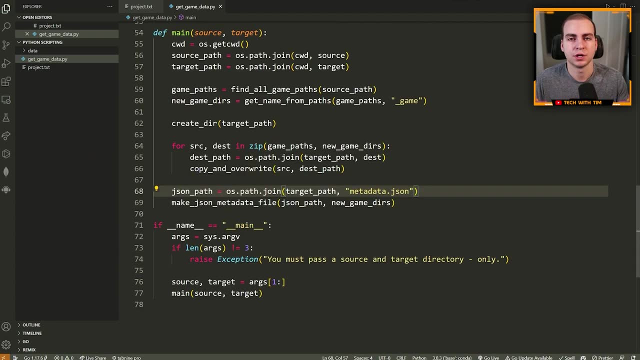 we have our game names and our number of games- Fantastic, So let me delete that, All right. Now that we have done that, I need to show you how we can compile this go code and how we can run the go code. All right. 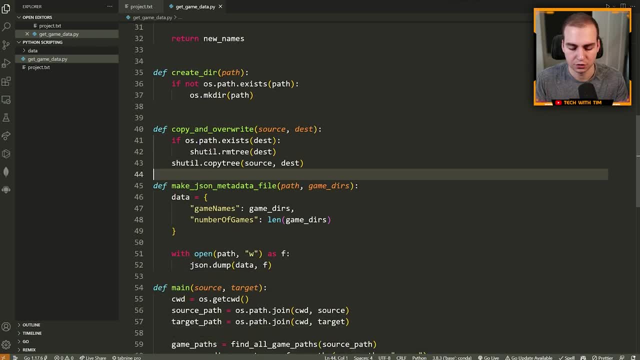 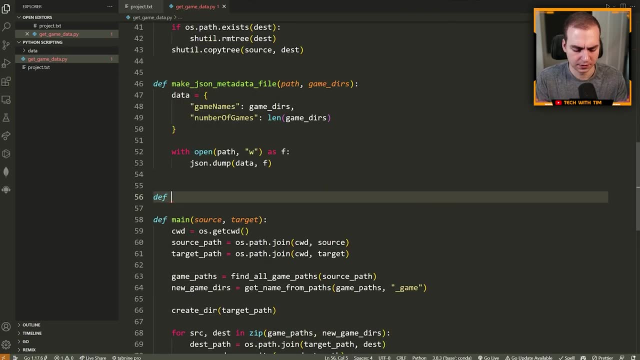 So let's write a function here that will allow us to compile the code inside of a directory. Now let me just space up my functions here So a bit easier To read. OK, and let's do it here. So define. this will be. 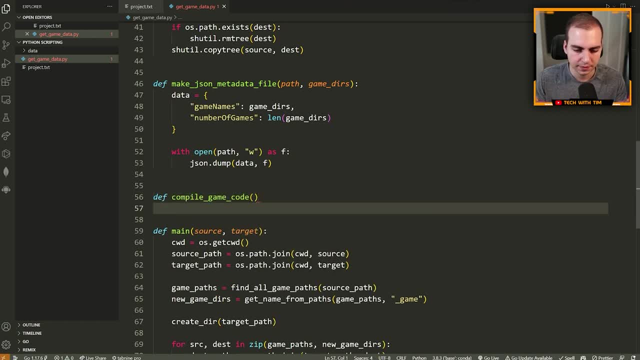 compile a game code Now. here we'll take a path which will be the path to the directory We want to compile the code inside of Now. what we need to do here is we need to locate or determine the name of the file. 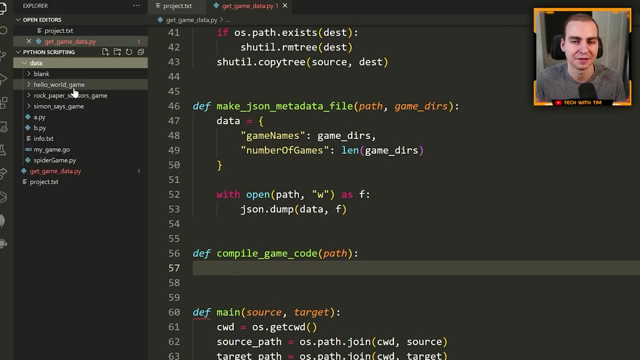 that we want to compile. You know, no pun intended or rhyme intended there, but you know what I mean. So we have main, we have code, we have file. Now, in this case we get hard code that, but we don't want to do that. 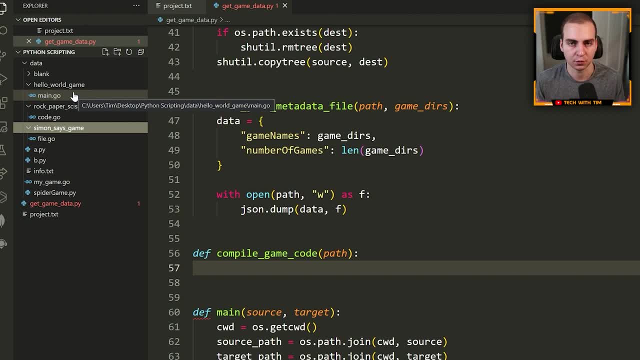 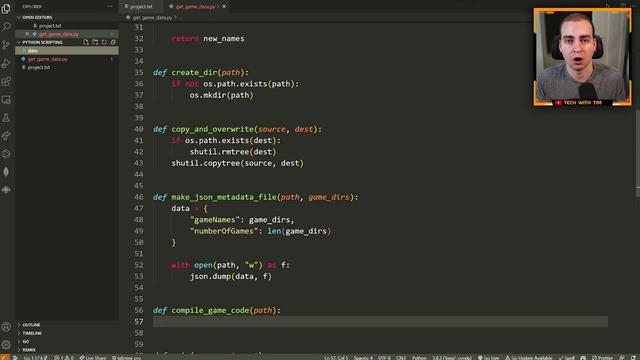 We want to have this dynamic So it works with kind of any go file, no matter what the name is. So essentially we're going to look through the directories of our games and we're going to search for any file that ends in dot go. 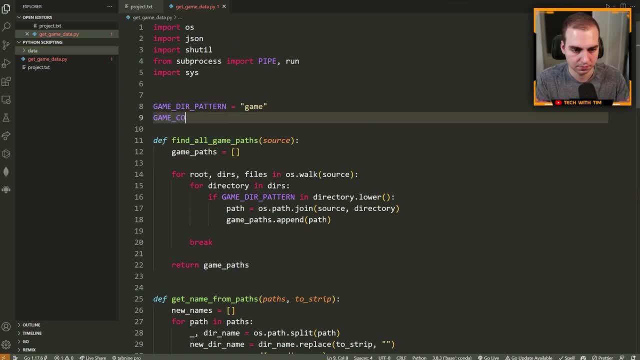 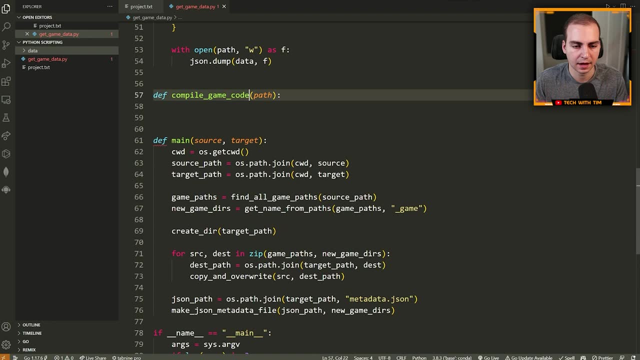 Right. So let's create a variable here and say game code extension, and I'll just make this dot go. So that's what we'll search for Now. if we find that, then we'll compile that code. Now we could compile. 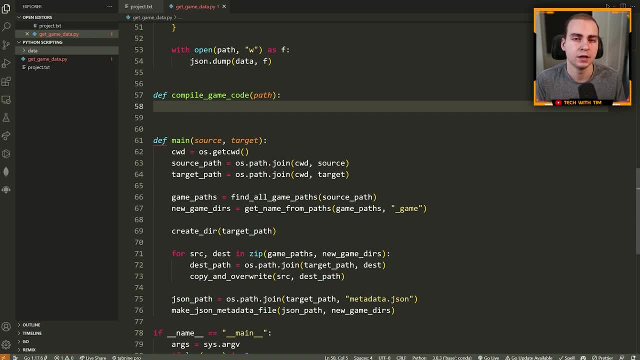 all of the files that have that name, or we could compile just the first one. In this case I'll just do the first one because we're assuming we only have a single code file in each of our directories. All right, So let's say code file name. 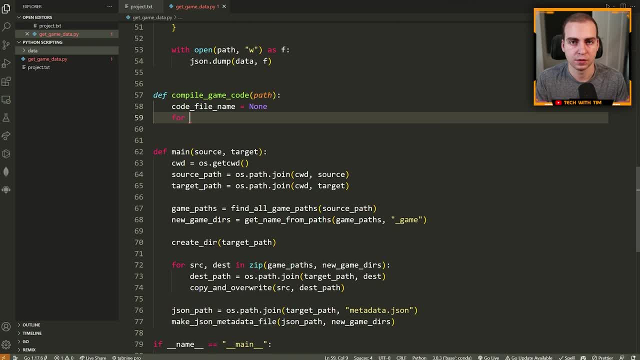 is equal to none. And then let's walk through this directory like we did before. So we're going to say: root, dirt files in OS, dot, walk our path. And this time we're only interested in the files. So I'm going to say: 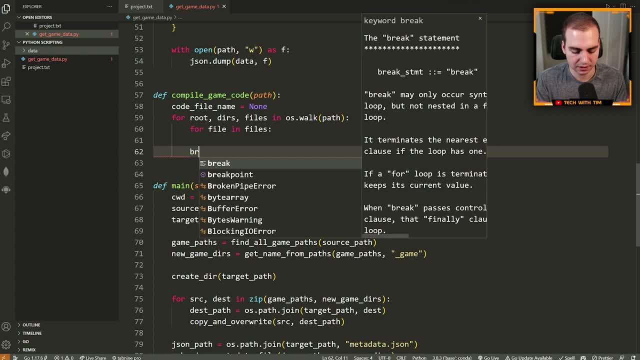 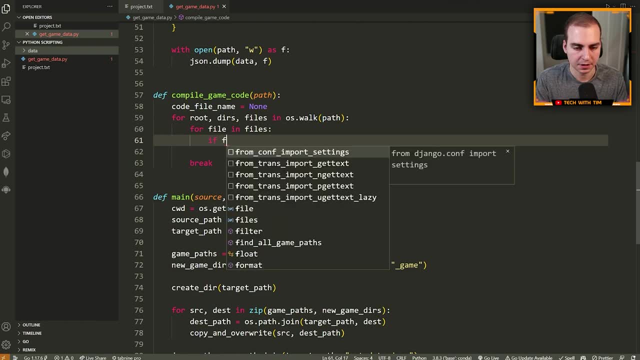 for file in files, And let's not forget to break here at the end of our for loop. So we only do this one time and not recursively. OK, so four files in files. I'm going to say: if the code, what did I even call this? 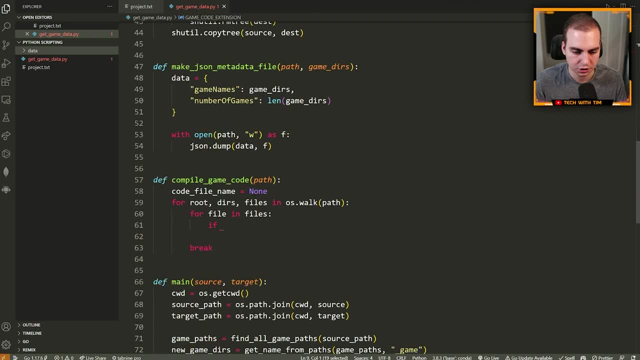 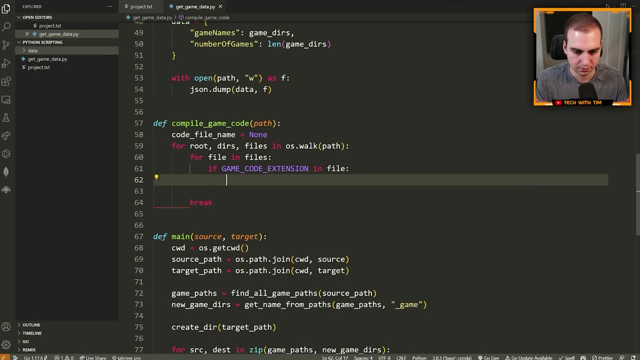 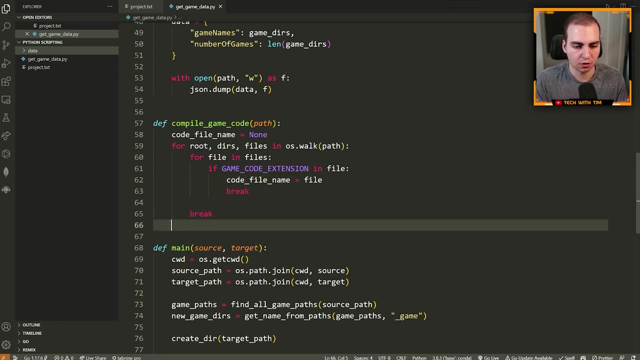 The game code. OK, game code extension. If the game code extension is in the file, then I will say my code to this. my code file name is equal to file and then I will break. OK, that's actually all we need. 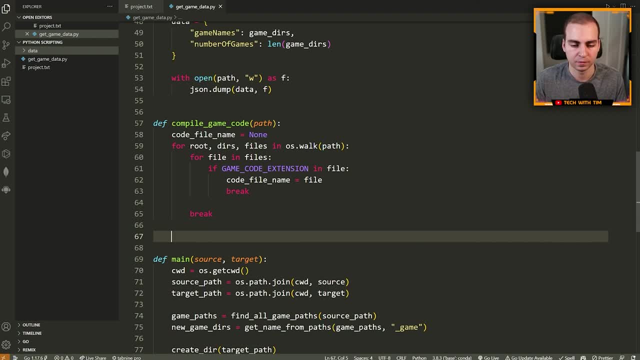 I know And fast there, but that's all. we need to determine what the name of our code file is. So we loop through all of our files here, right So for file and file, and we say OK, if this dot go extension. 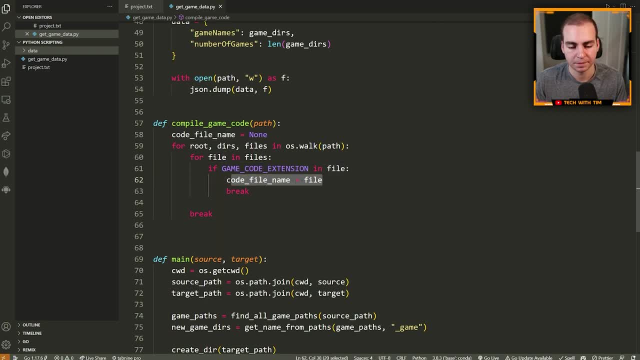 is associated with the file, then we'll say: code file name is equal to five, and then we'll break, which means we'll just find the first one. We don't need to continue looking Now. what I just realized, though, is that this could be a little flawed. 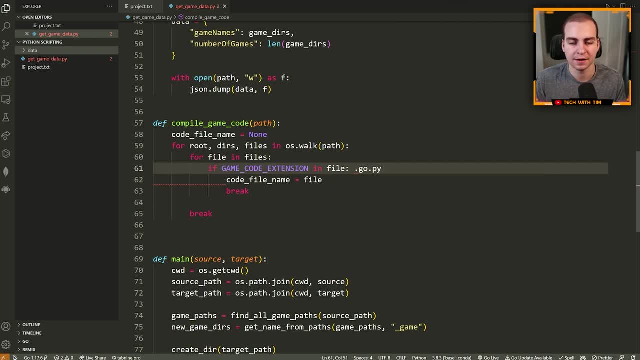 because I could technically have a file that's like dot go, dot pi. I know that would be a weird name, but that wouldn't be a dot go file, That'd be a Python file, Right, Well, I think that would be a Python file. 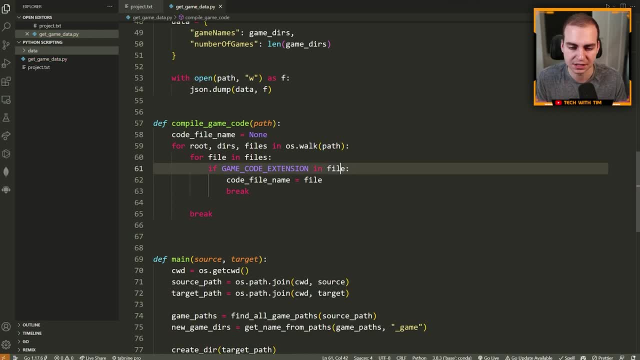 but it would be a bit weird either way if we had something like that. So what I'm going to do instead is use a little bit of a better way of doing this. I'm going to say, if file dot ends with, So I'm going to check. 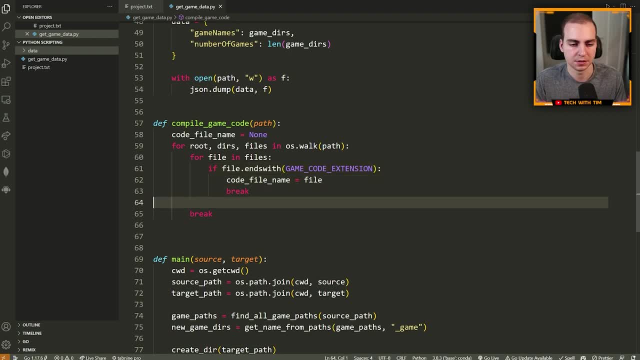 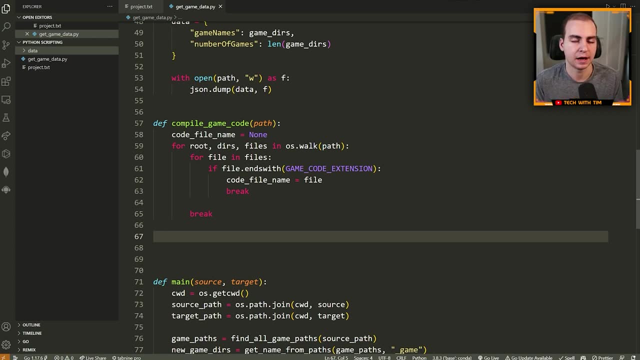 if this is at the end of the file. I think that's a better way to do this. check OK, perfect. So now what I'm going to do is I'm just going to make sure that we did have a code file, If we don't have one. 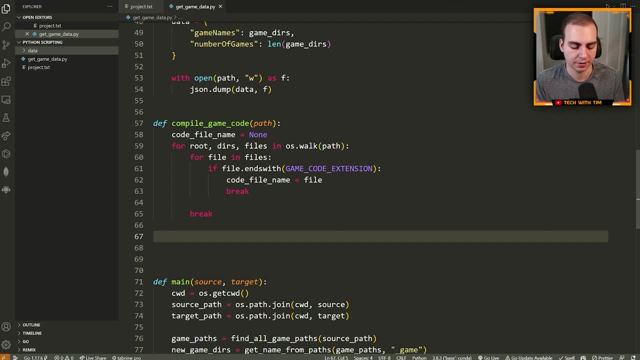 I'm going to return. If we do have one, then I'm going to run the command to compile this. So I'm going to say: if the code file name is none, then just return, just so that we don't get an error when we try to compile a file. 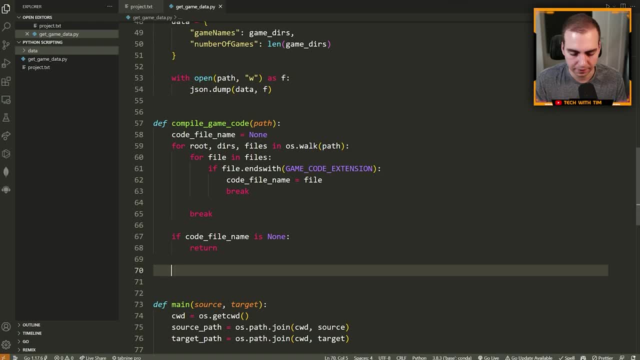 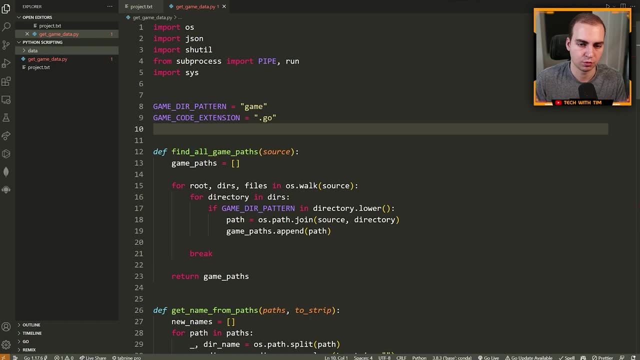 that doesn't exist. Now we need to actually compile the file. So the first thing I'm going to do is say my command is equal to, and then I'm going to make a variable up here which will be my compile command. So I'm going to say a game. 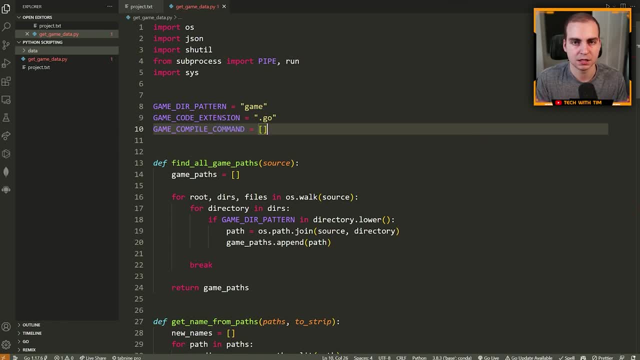 compile command. Now, the way you write these commands is just in an array of- I keep saying array- and in a list of strings that represent the commands that you need to run. So it's going to go and then build. So this is the command: go build. 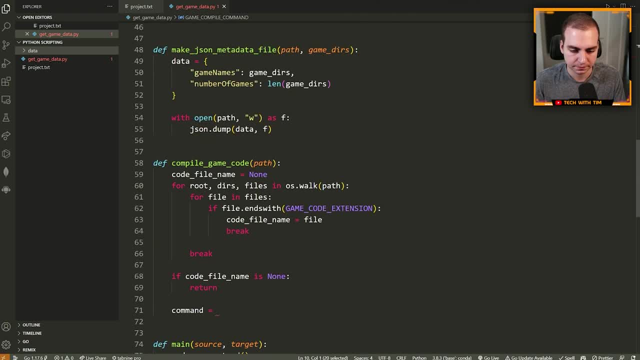 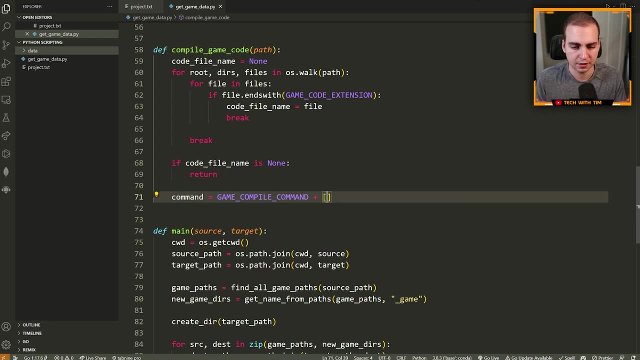 than whatever the name of the file is. So this is my like base command. So I'm going to say my command is equal to my game compile commands plus, and then I'm going to put another list here and I'm going to add inside of here: 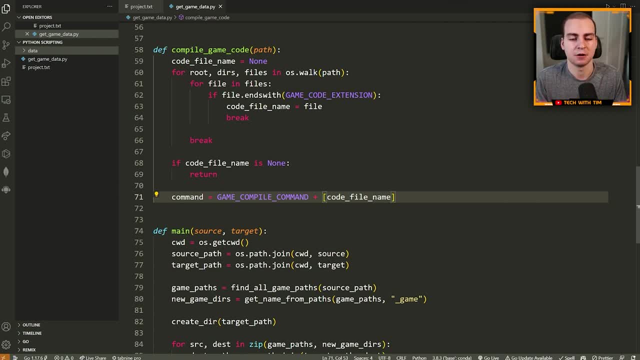 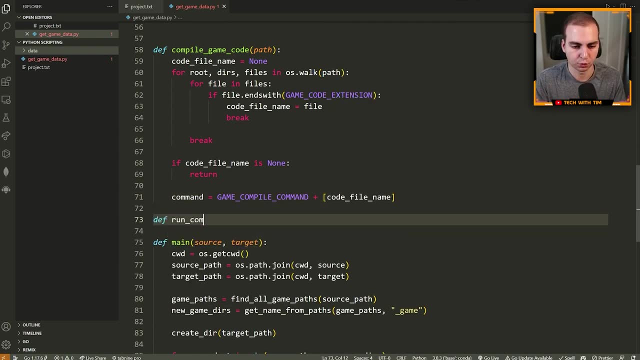 the code file name. Now, what this will do is make the command be go build and then, whatever the file name is, then I can pass this to a function that I'm going to write, which will just run any any command that I pass it. 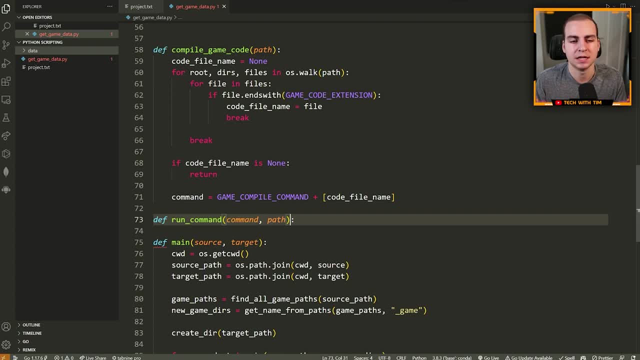 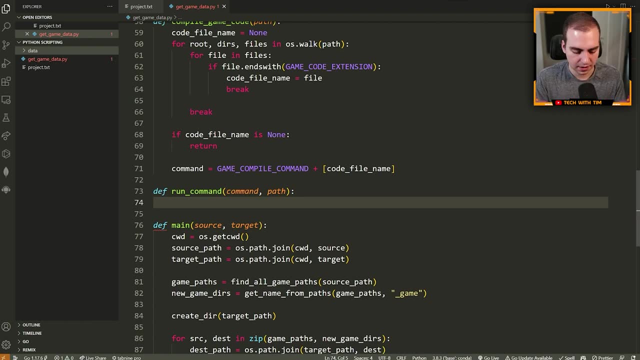 So we're going to say: run command. We do actually need the path that we want to be running this command from. OK, so now I'm going to say that our current working directory is equal to OS dot get CWD. Is that? is that what it is? 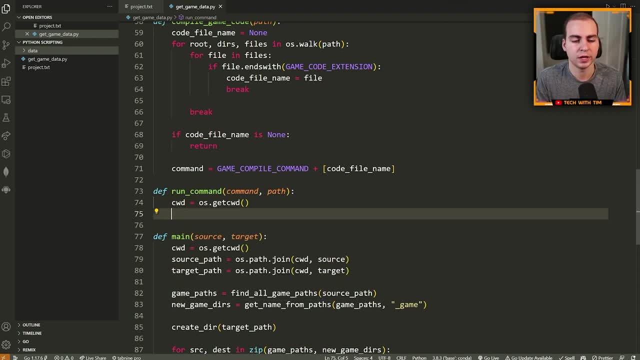 Get CWD. Yes, that's correct, And I'm going to show you how we change our working directory into this path. The reason for that is that I need to run this command. Well, I don't need to, but I'm going to run this command. 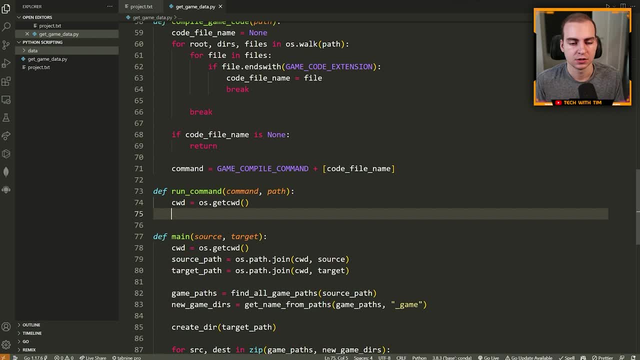 directly in the directory where our game code is. So, rather than being in the directory where my Python script is run, I'm going to change into that directory, run the command and then change back to a different directory. just to show you how you do that. 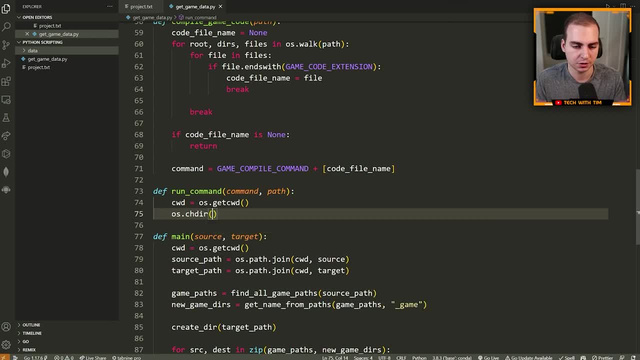 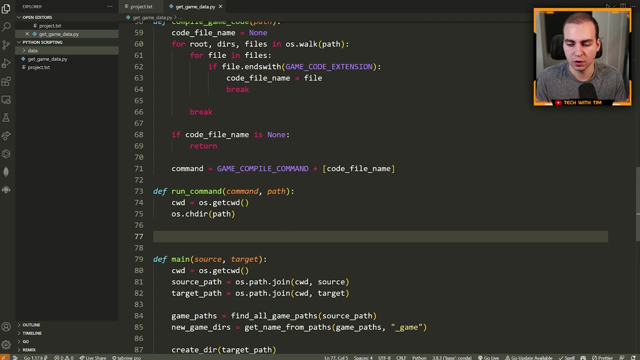 So I'm going to say OS, CH, der, which stands for change directory. I'm going to change into the path directory. Then I'm going to go and run the command. Now, to run the command, we're going to use the sub process command run. 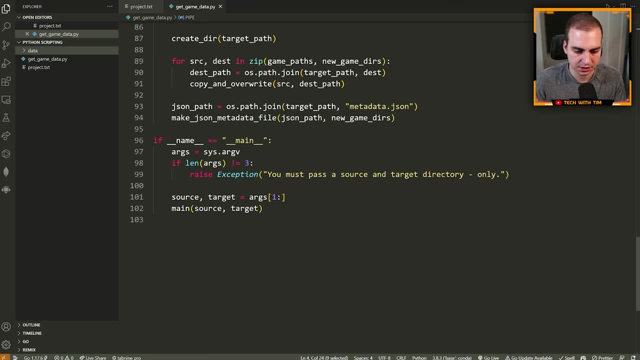 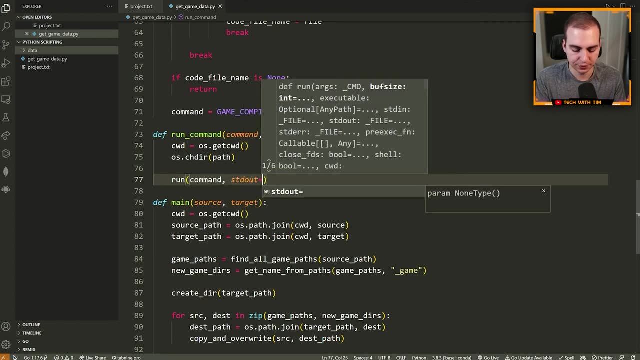 which I believe I import it from up here. Yes, I did So. we're going to say Run and we're going to run our command and we're going to say: our standard output is equal to pipe and our standard input is equal to pipe. 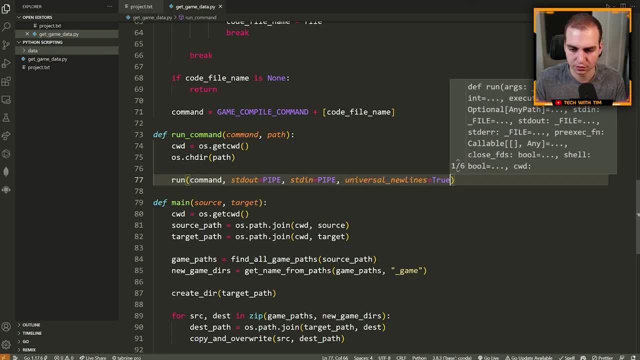 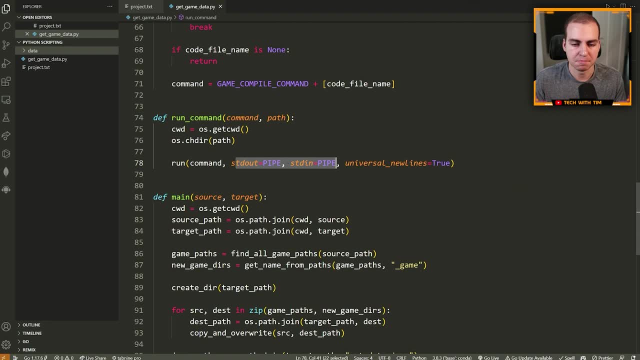 And I'm going to say universal new lines is equal to true. Now, this is where the command gets a little bit complicated, right? You know what does all this mean? Well, the standard output in the standard input is the location where the command is. 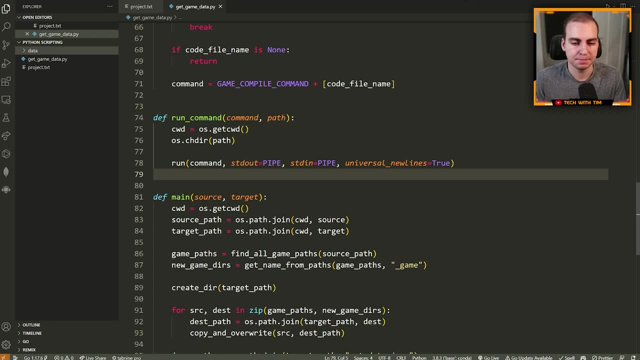 accepting input and spitting out the output. Now, pipe is kind of this special thing that we can use that makes a bridge between our Python code and the process that we're using to run this command. Now I'm not really going to explain it. 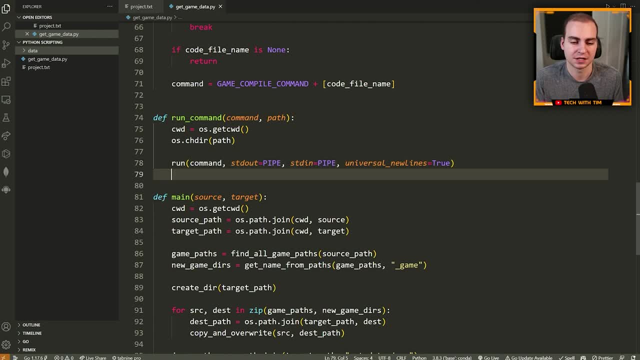 more than that, but just understand that. that's why we're putting it here. It essentially allows us to communicate between the process that can actually run this special command, because this command is not a Python built in command right Like this is a command. 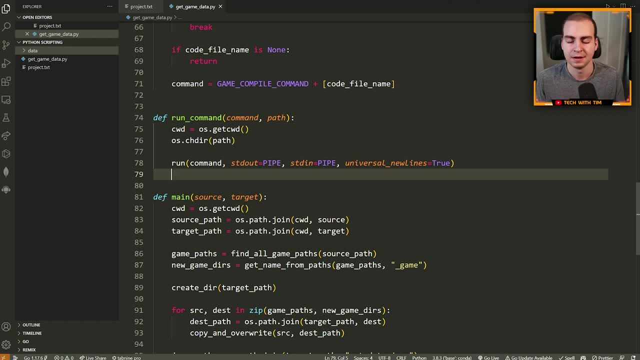 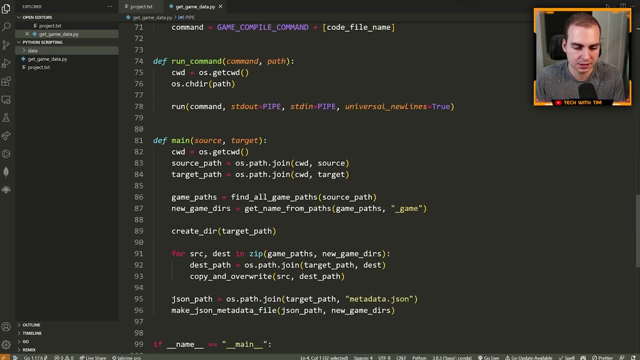 we just run in our terminal or in our command prompt. Again, you don't have to understand it. Maybe that explanation was good, Maybe it wasn't, But this is how you do it. You import, run and pipe from sub process. You pass the command. 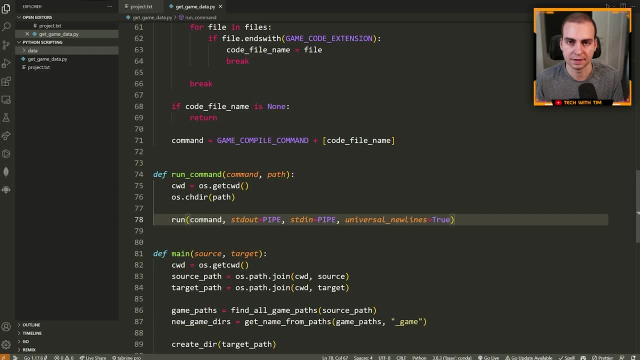 Again, the command is just going to be an array of all of the different words that are in that command, or a list of all of the different commands, And then, if you wanted the result, it will be given to you in this result variable. 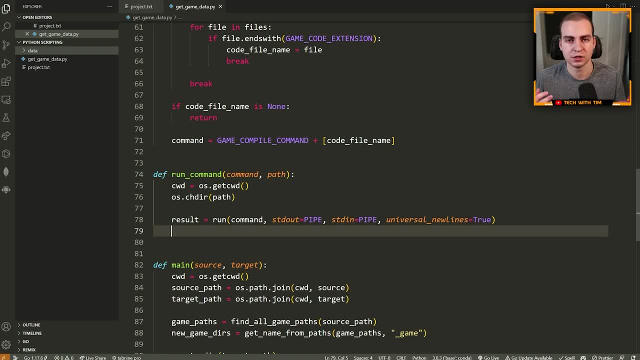 So you could print out the result, You could read it in as a JSON object, blah, blah, blah. You could do whatever you want and you could see what that result is. And in fact we'll print out the result, just so you can see. 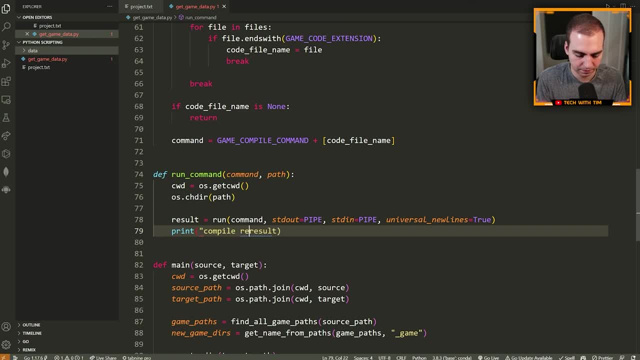 what it looks like. So I'll say: Compile result like that. OK, now the last thing we'll do, just as good practice, is, we're going to change our directory back to the current working directory. we were in before we ran, or before we changed. 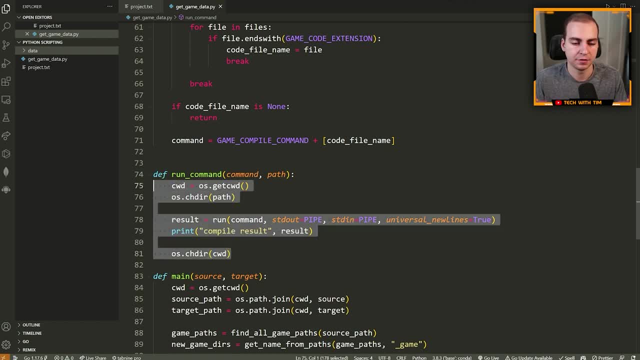 directories into this path, just to make sure when we run this command another time we don't get any potential errors. OK, so we got the working directory we were in changed into this path directory, ran the command and then we went back into. 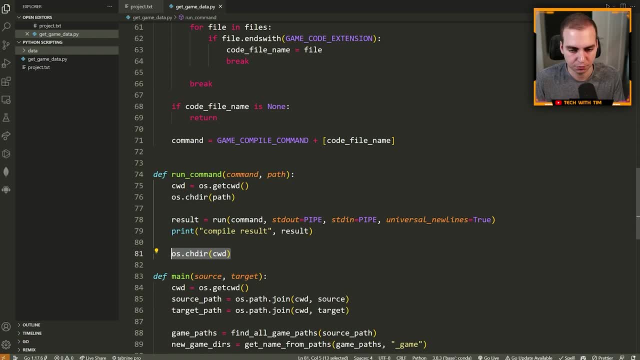 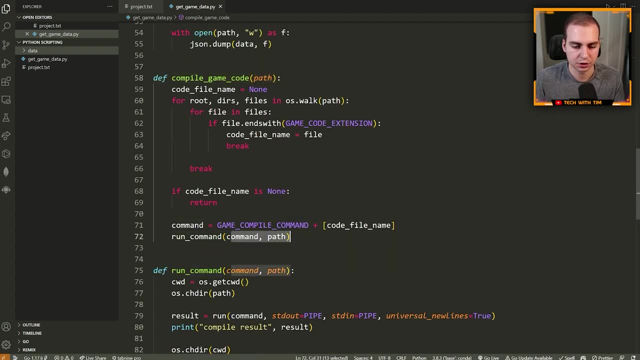 whatever the previous directory was, just that we don't have any potential problems here. Now we need to call this function. So we'll say: run command and command and path. That's actually fine. We can just pass those values, Great. So now where do we call? 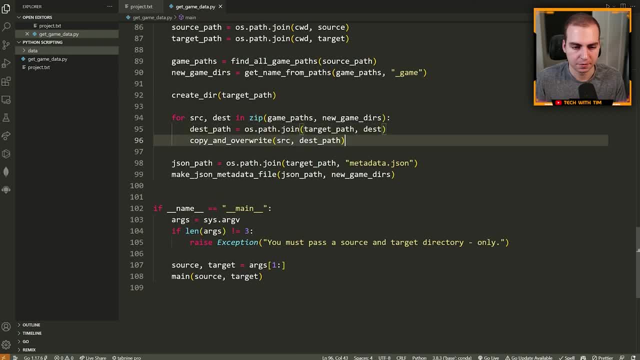 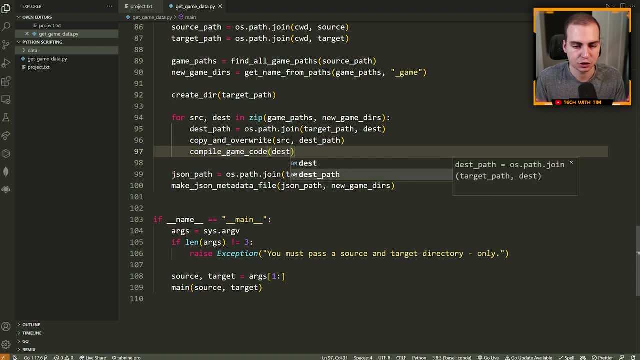 our compile game code function Well, we're going to call that from inside of our copy here. So I'm going to say compile game code and I will compile game code in the destination path, because once we've done the copy and overwrite, once this is finished. 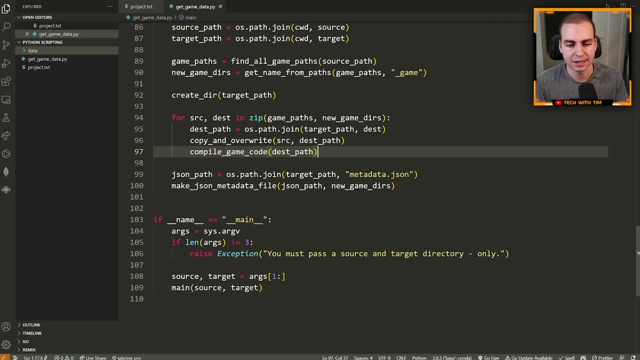 now that directory exists, let's compile the game code, then move on to the next directories. So at this point the project is pretty much finished. Let's run it, though Make sure it works OK. compile result. compile result. 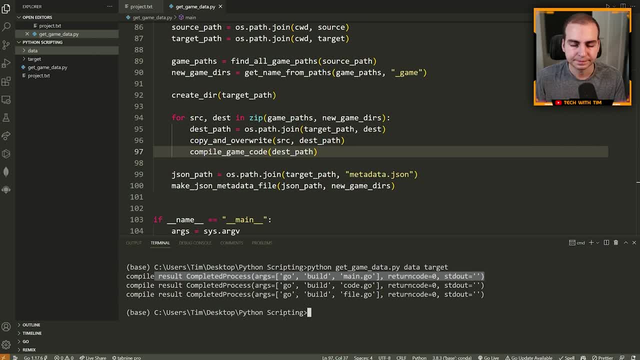 and notice it gives you kind of this like result, object right. I'm not going to again kind of dig into exactly how this works, but you can see that if you wanted to look at the standard out then it would be STD out from this compiled process. 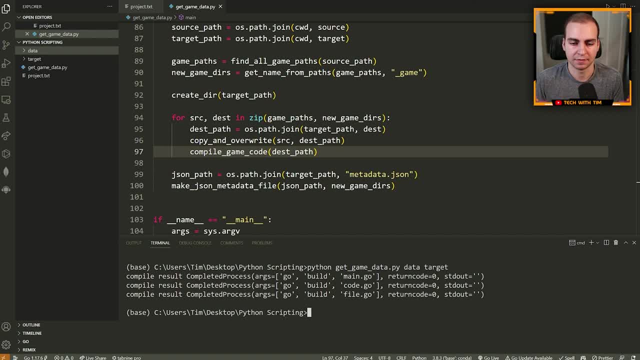 We're sorry, not compiled. completed process, And if this had any result- like if there was an error- you'd be able to see it there And the return code would most likely be an error return code as well. Now let's look at target here. 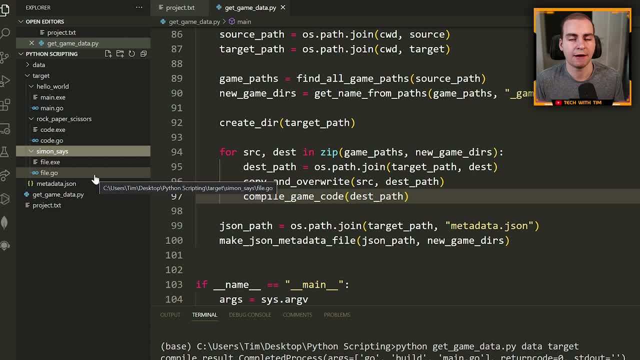 So we have target, We have Hello World. And now, notice, inside of my directories, I have my compiled code, right, I have main, dot exe, code, dot exe, file, dot exe, et cetera, If you were on Mac or Linux.